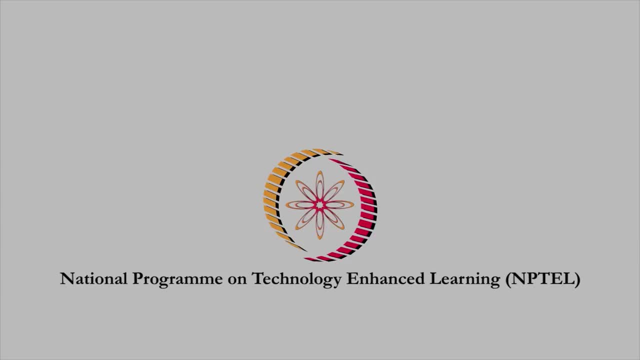 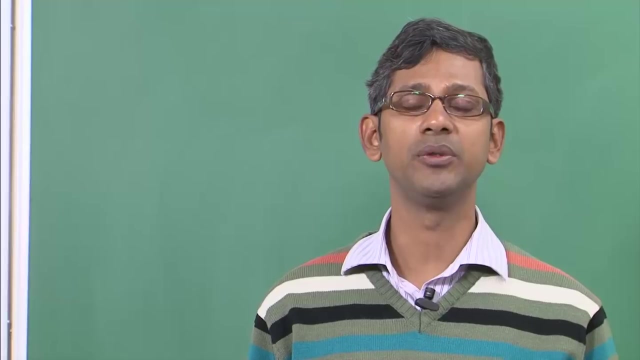 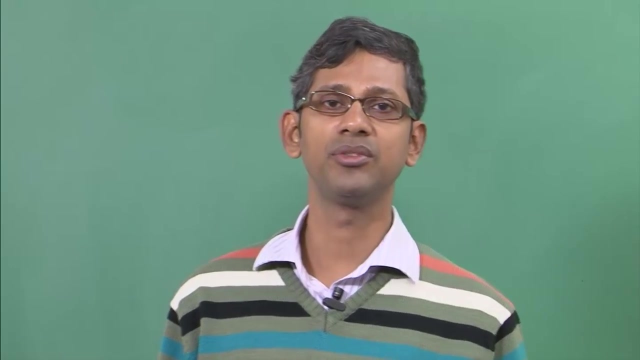 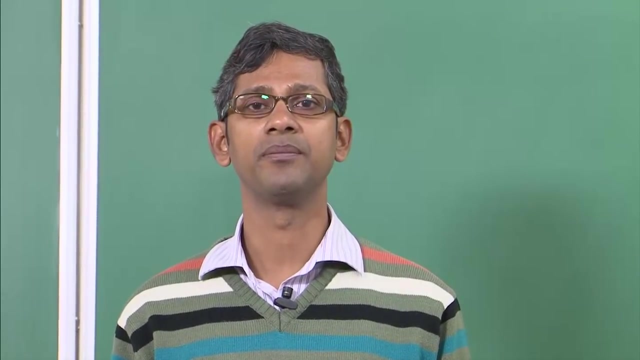 Hello everyone. today we are going to start a new topic, that is, eutectic phase diagrams. I think I have discussed about the binary isomorphous phase diagrams in details and you have gotten fair idea about the different facts of this phase diagram, The binary isomorphous phase. 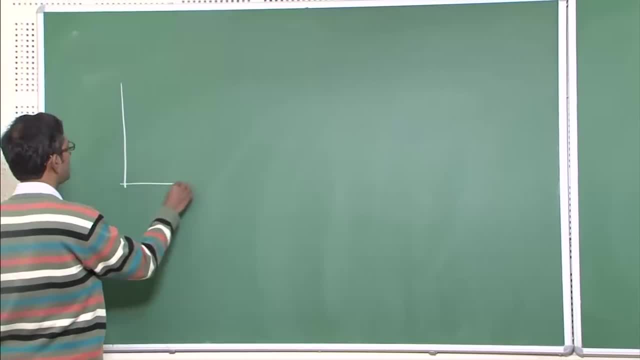 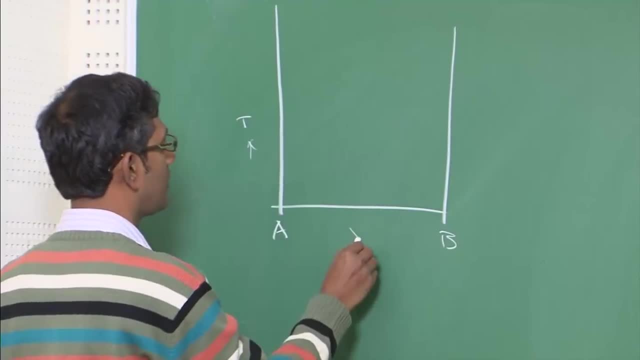 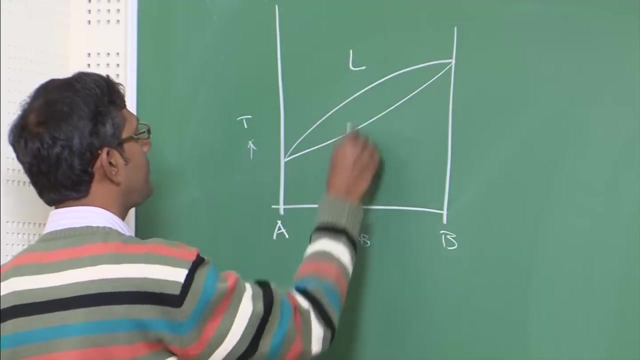 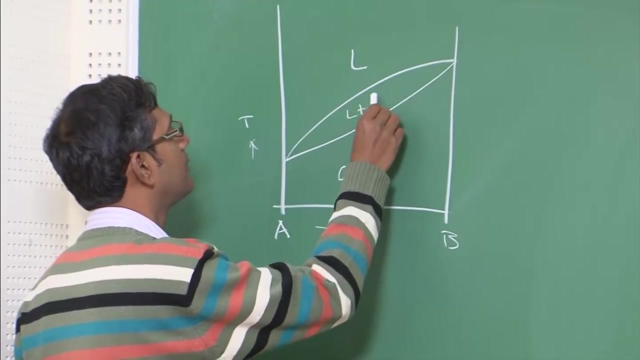 diagram looks somewhat like this: If I take a binary system- A and B- and plot temperature versus composition, then I get a phase diagram which looks like a lens. This phase diagram has three zones- Solid and solid phase- and these two zones are surrounded by liquid plus solid or liquid. 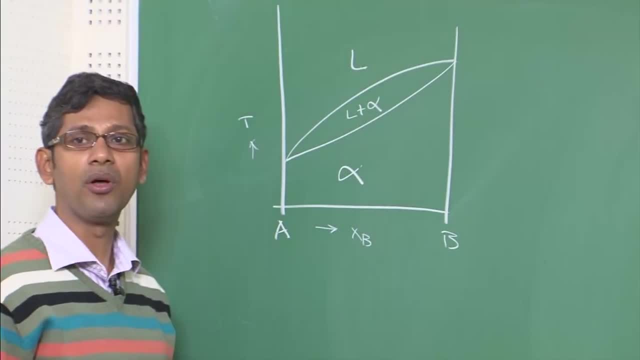 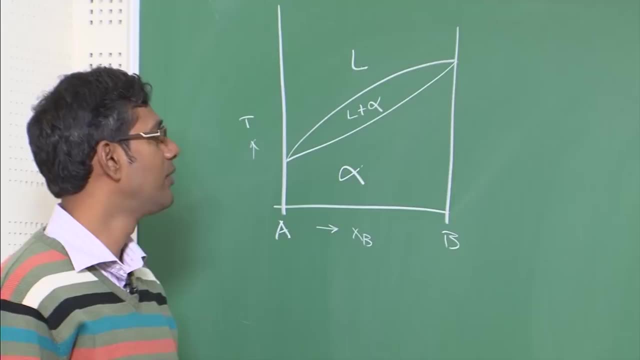 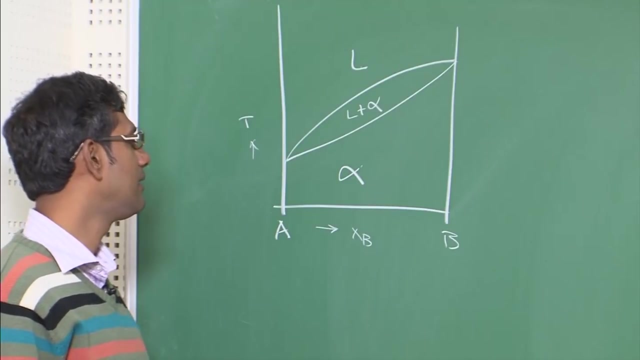 plus alpha. Now, such a kind of phase diagram is possible only under certain conditions, and these conditions are very strict. So first condition to be satisfied by the two components A and B is that the size difference, or the atomic size difference of between A 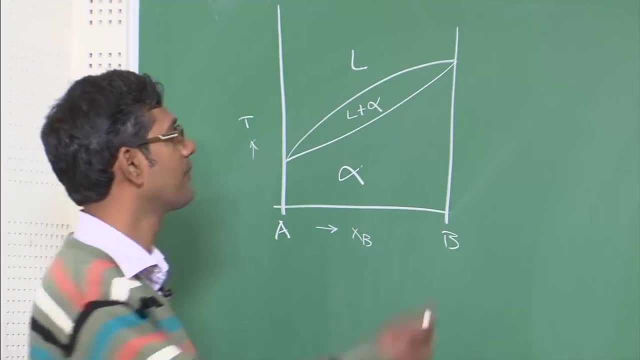 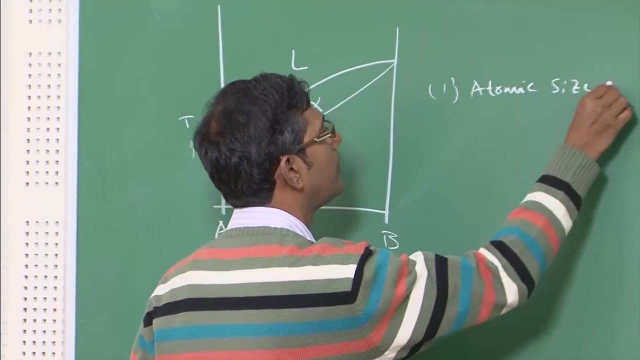 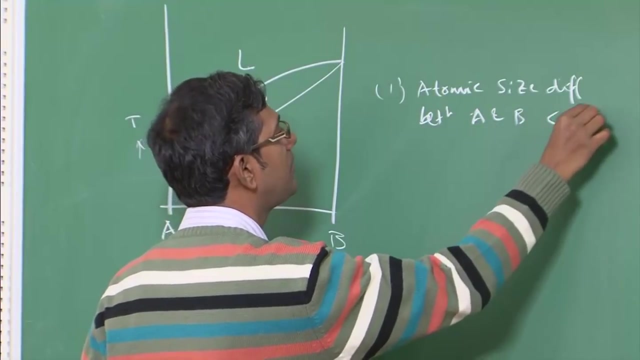 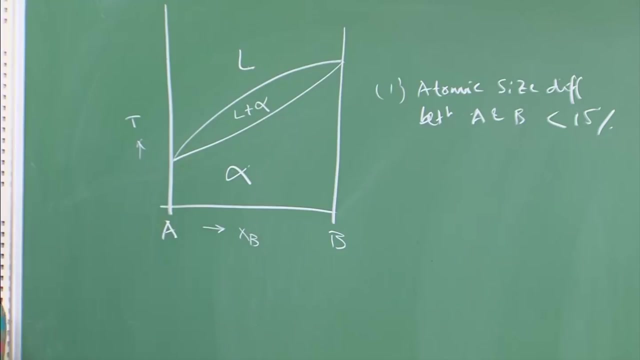 and B should be less than 15 percentage. So that means the atomic size differences between A and B should be less than 15 percentage. This is the first condition to be satisfied by the two components, A and B, for such a kind of phase diagram. Second condition to be satisfied: 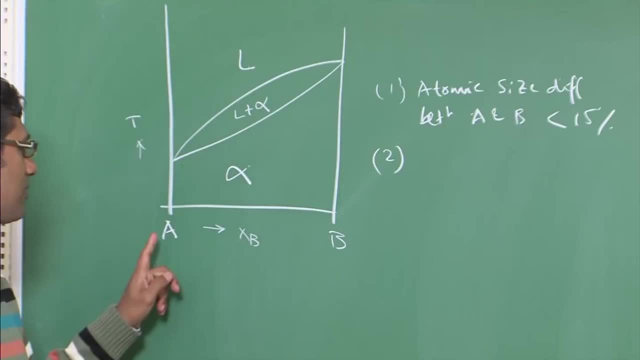 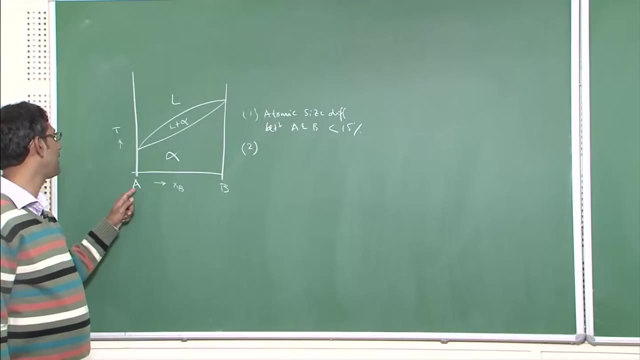 is that they must have similar crystal structures, Like A and P should have cubic crystal structures with themselves or hexagonal crystal structures Similar means. A can have FCC, B can be BCC or A and B. both can be FCC or A and B both. 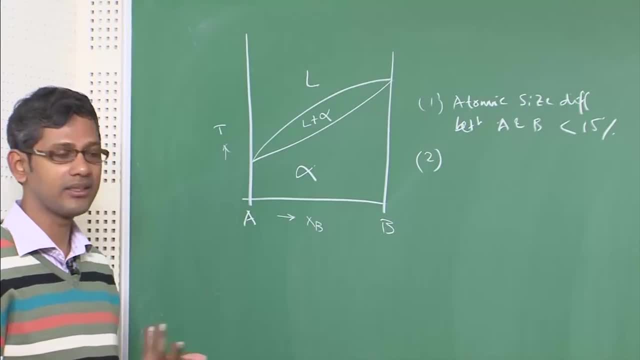 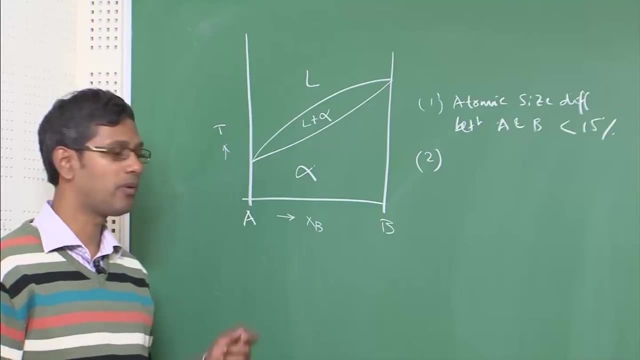 can be BCC or A and B. both can be hexagonal. any other crystal structure, by the way, Like germanium and silicon, both have diamond cubic structure. Then bismuth and antimony both have: one is a Rombaud, other one is a hexagonal crystal structure. So they all form binary. 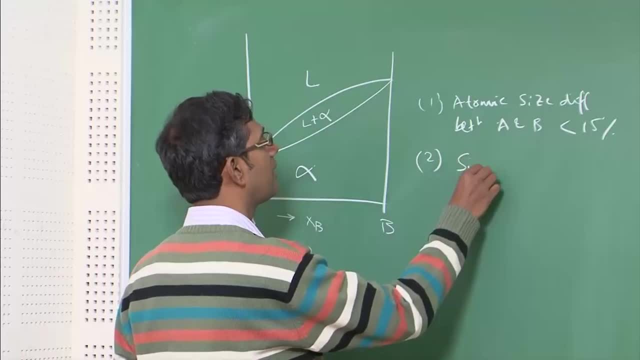 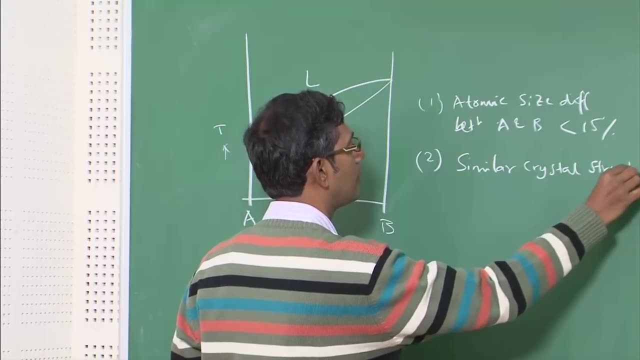 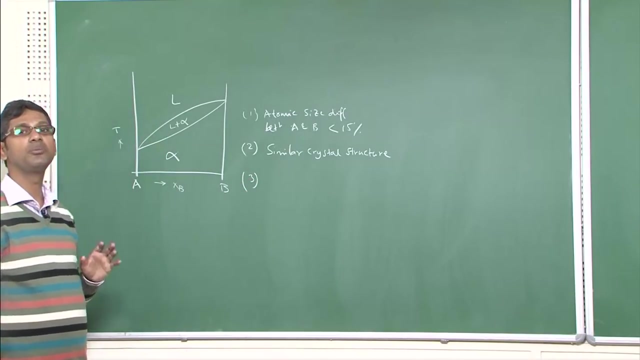 isomorphous phase diagram. So similarly, if I take a binary system- A and B- and plot temperature versus composition, similar crystal structure is the second condition to be satisfied. Third thing to be satisfied is that the electronegativity difference between A and B should be very. 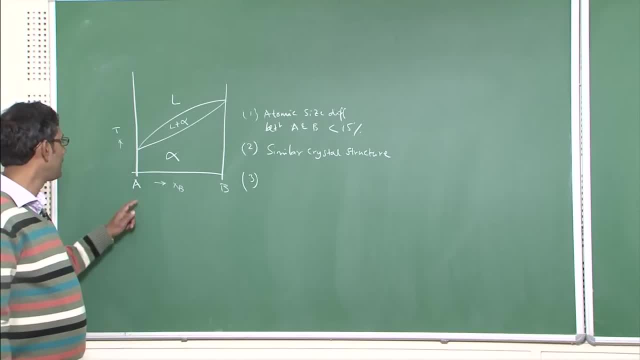 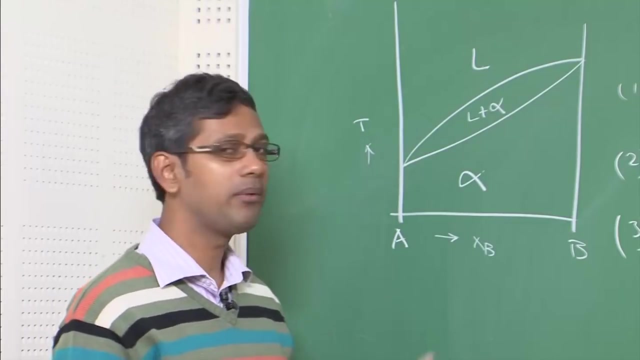 small. Why? Because if the electronegativity difference between these two components are very high, then there will be compound formation. Suppose sodium and chloride. if you consider Then what will happen? They have huge difference of electronegativity, so it will form sodium. 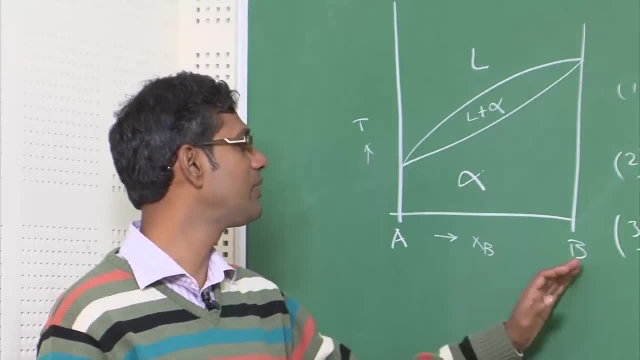 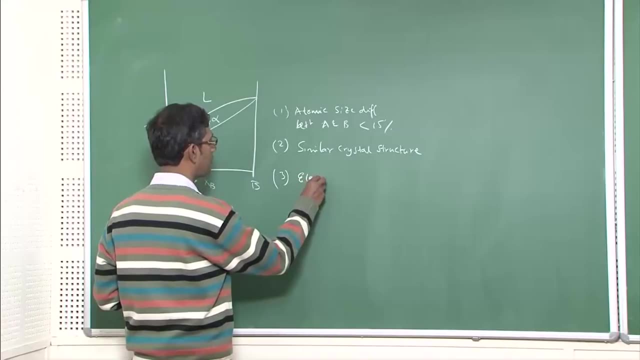 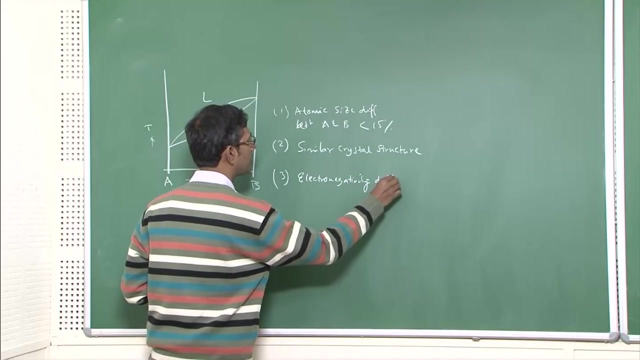 chloride structure. So that means electronegativity difference between the two components must be very small, as small as possible to form isomorphous system. This is the third condition to be electronegativity differences where it is very small. The fourth: 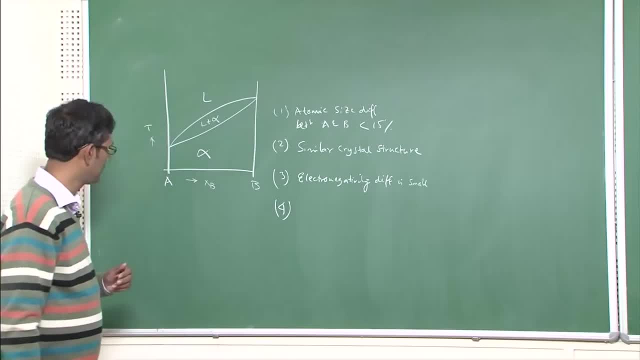 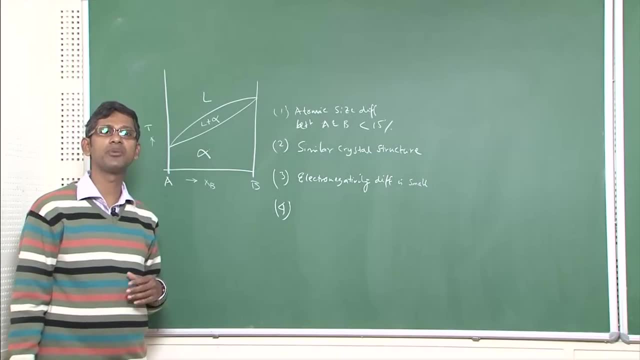 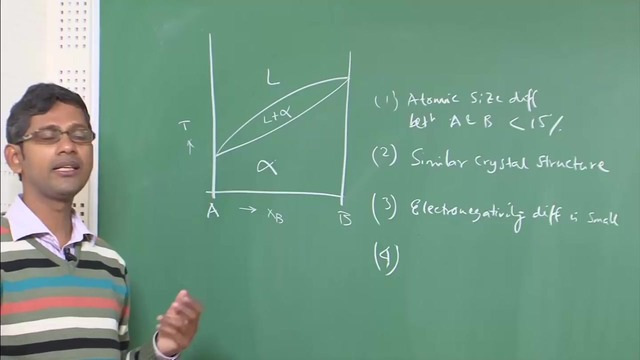 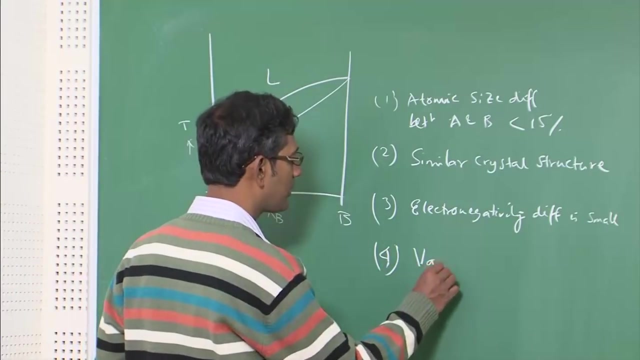 condition to be satisfied is that the valency of these two elements or these two components should not be widely different. Suppose: consider an element between- I will tell- copper and nickel. The valency difference between these two elements are very small, so therefore valencies will be similar or almost same. 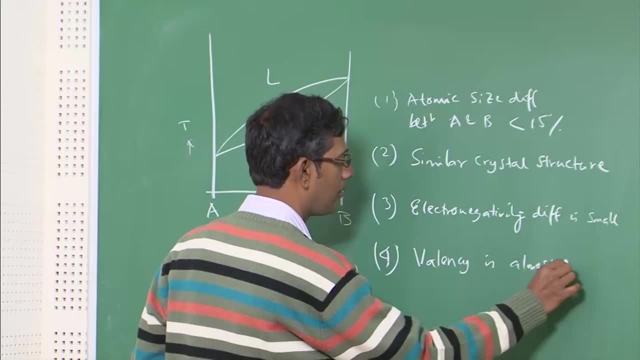 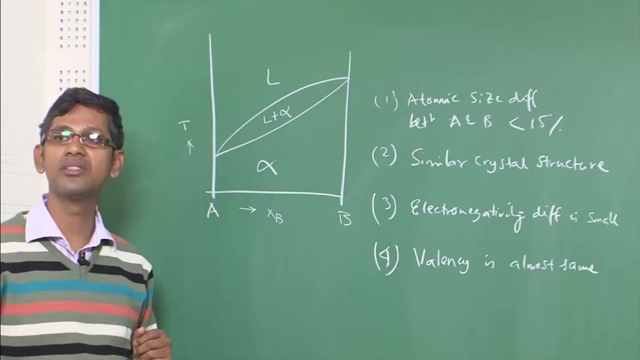 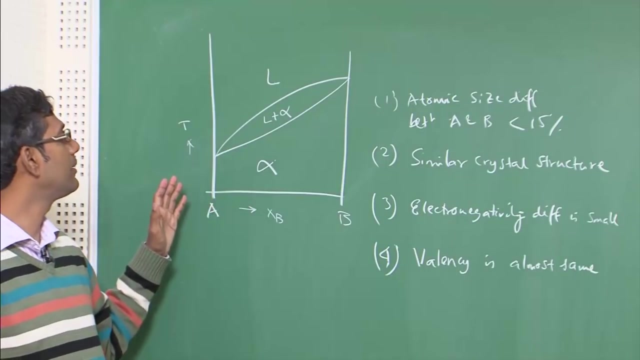 So, but you know these are the conditions to be satisfied to form and binary isomorphous system. It is true for ternary isomorphous system also, but for the sake of simplicity we have considered binary. So now you know these conditions are developed by scientist. 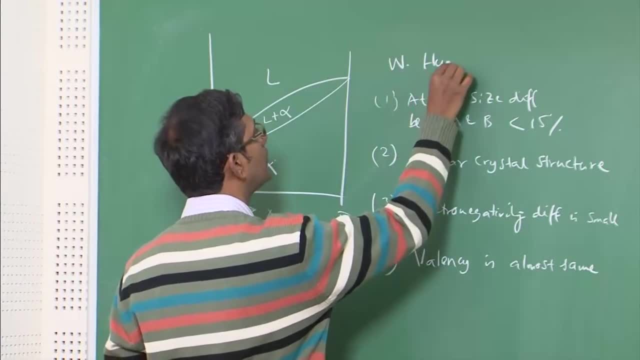 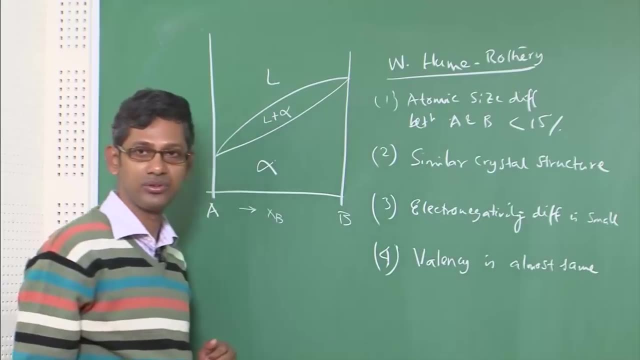 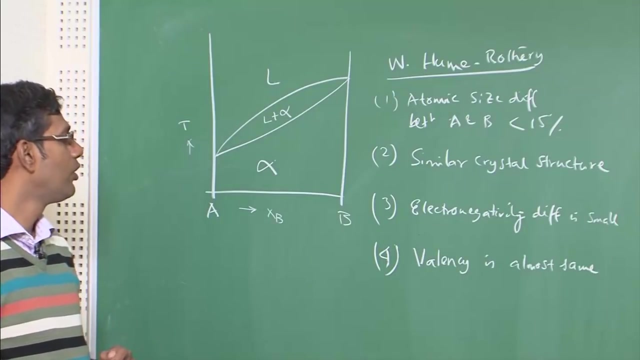 known as William Hume Rothery from Oxford University Long back, So these are called Hume Rothery. rules for formation of isomorphous phase diagrams or continuous solid solutions, but it is not possible always to satisfy all the conditions, So there are many elements. 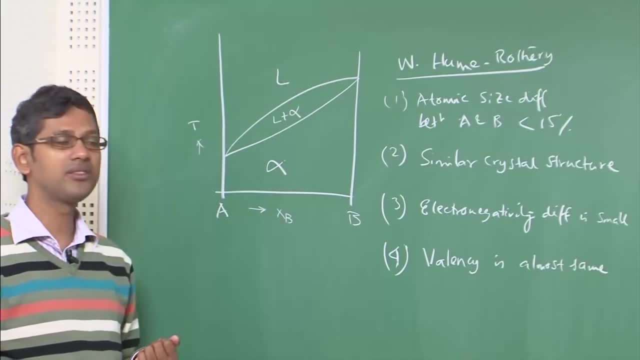 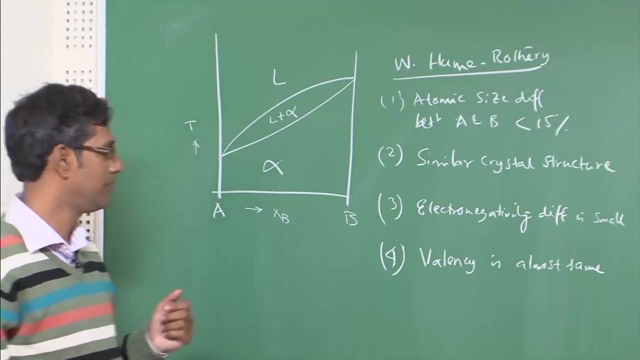 which will not satisfy. So for those elements, there will be deviation from this phase diagram, and once such deviation is eutectic. What is that? If I considered an eutectic phase diagram? Simplest one, Simplest one. 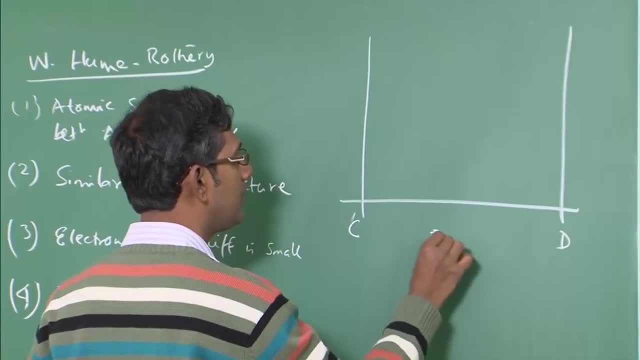 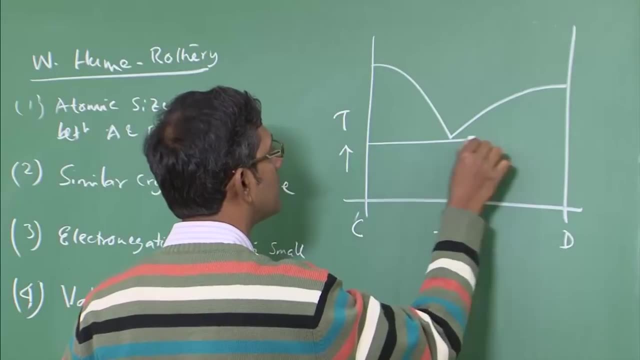 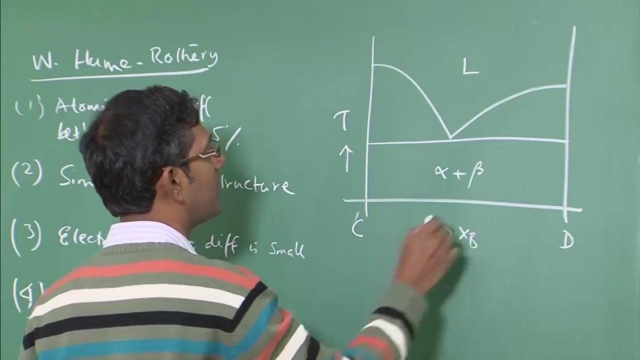 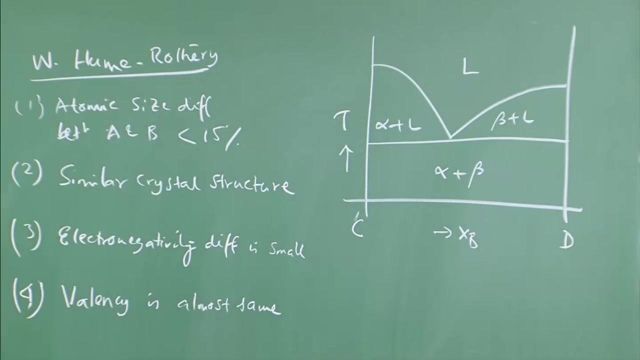 1 between, suppose, a component C and D. It will look like this: This is again liquid solid, alpha plus beta. There are two solids. I am just marking, but I will explain everything to you. So what do you see here? You see here that obviously the liquidus here as liquidus, 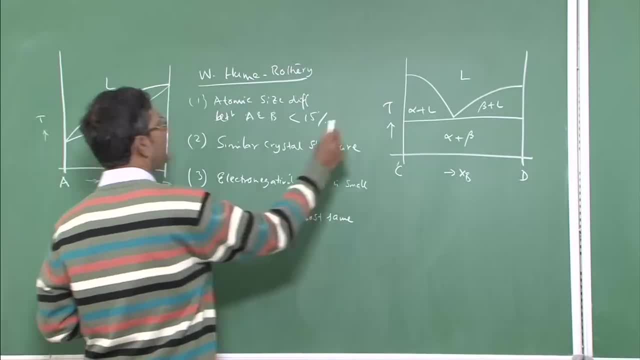 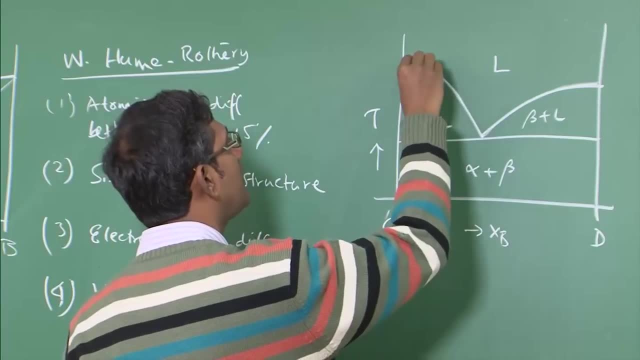 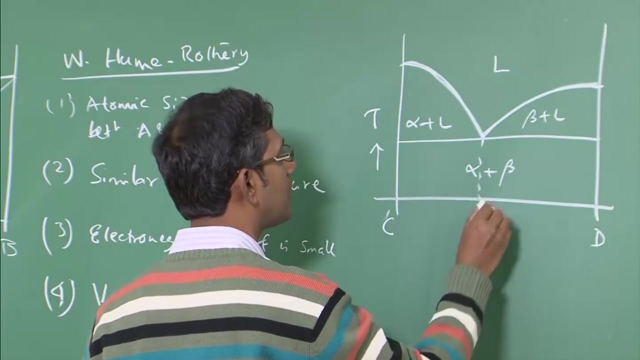 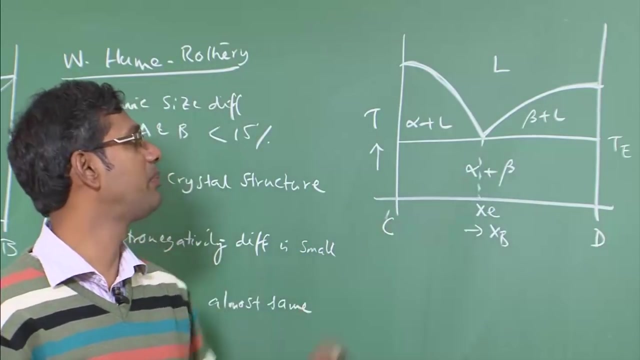 here is this line, this curve. Here the liquidus is this one, and you can clearly see the liquidus as a dip at certain composition, which is given by this, and certain temperature, which is given by this. So this is as basically this kind of dip if it is present in a phase diagram. 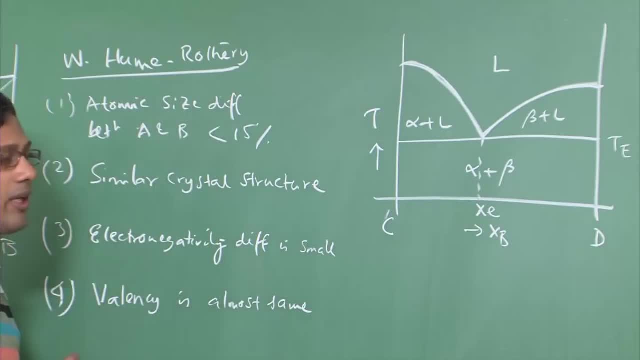 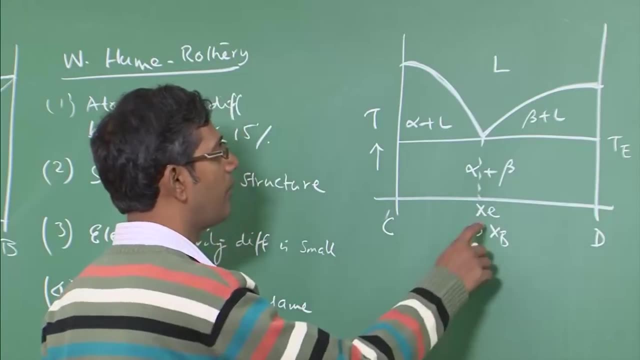 we call it as a eutectic phase diagram. Why we call it eutectic phase diagram? Because it is a phase diagram. Why we call it eutectic phase diagram? Because if you have such a kind of dip at a temperature equal to Te composition. 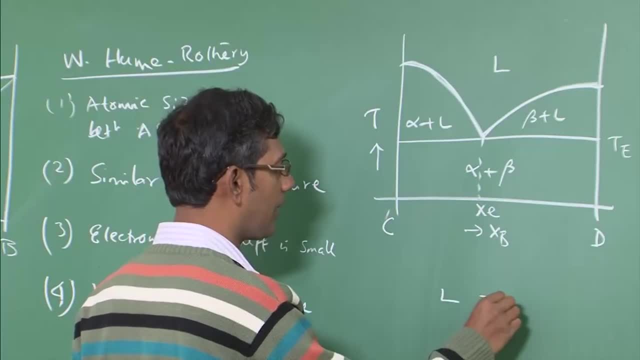 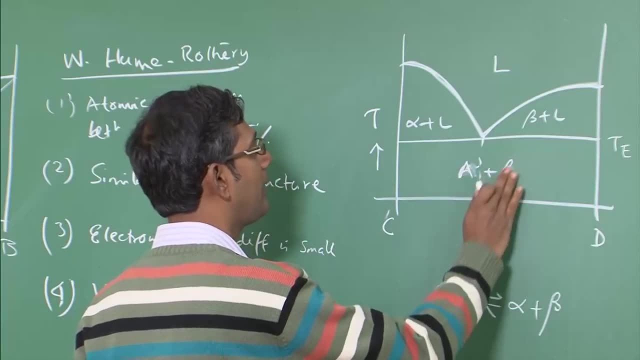 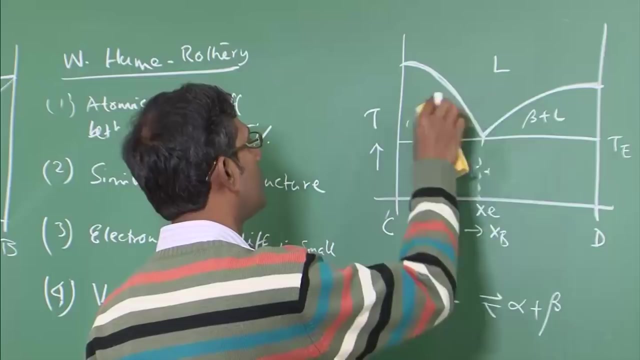 Xc, so that means at the temperature liquid undergoes a reaction during cooling leading to formation of two solid phases. here It will be A and B. This will be A and B. Let me write down, otherwise you will be getting confused, because these are two pure components. 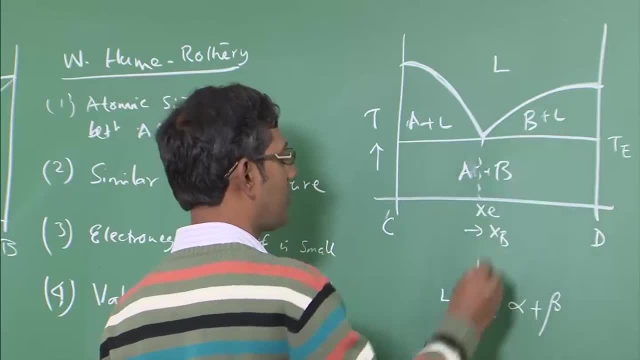 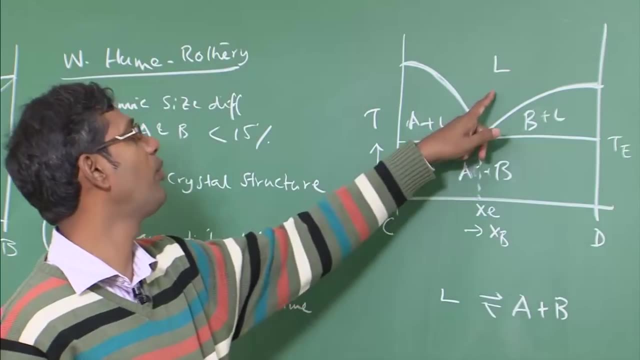 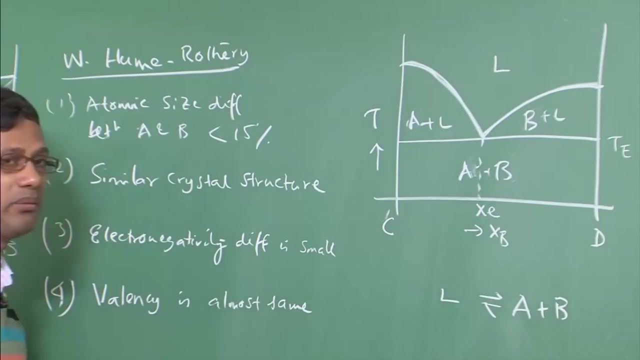 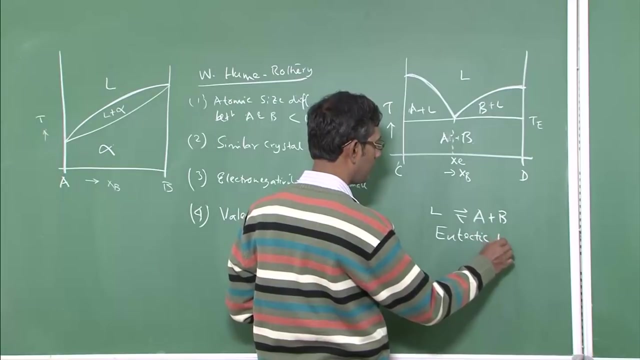 therefore A and B. Please make this correction So liquid going to A and B at. this kind of reaction will happen when you cool down from high temperature to low temperature through this composition, So liquid will separate into two solid phases, A and B, and this is known as eutectic reaction. 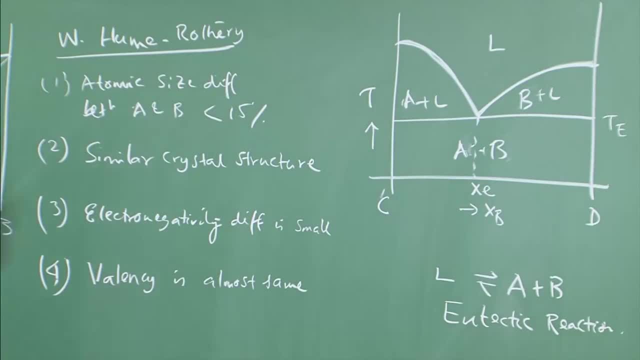 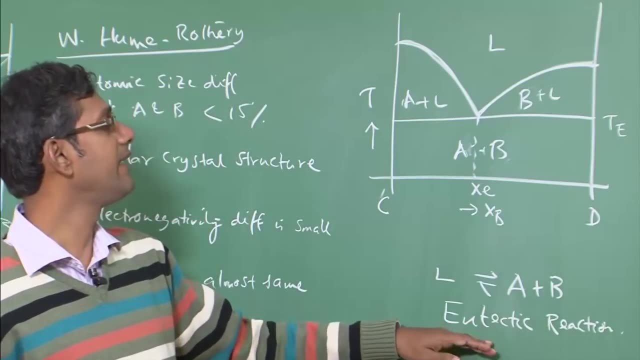 This is known as eutectic reaction. Eutectic reaction, Eutectic reaction. Eutectic means easily meltable. in the Greek literature, Eutectic means easily meltable. That means anything which melts very easily is known as eutectic. Why? Because, if you 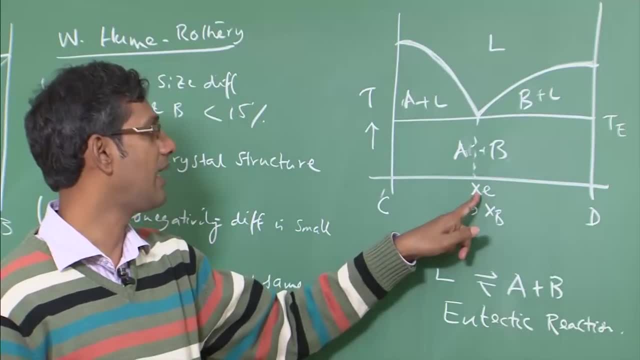 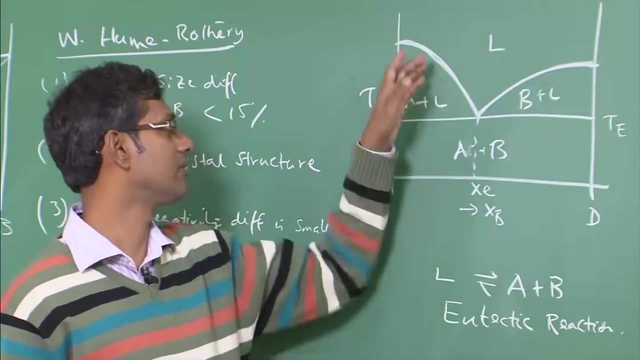 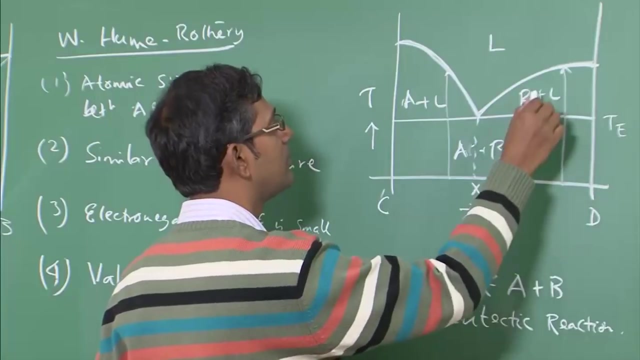 look at this diagram. this composition at Xc melts at temperature Te, but any other alloy composition will melt at high temperature. If I consider this alloy, the melting temperature of this alloy is this, or this alloy means this alloy is this, which is higher than Te. 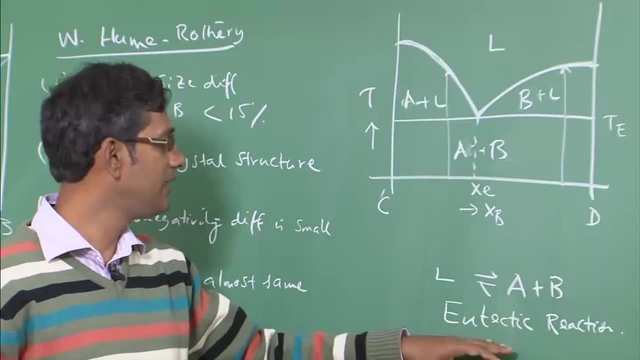 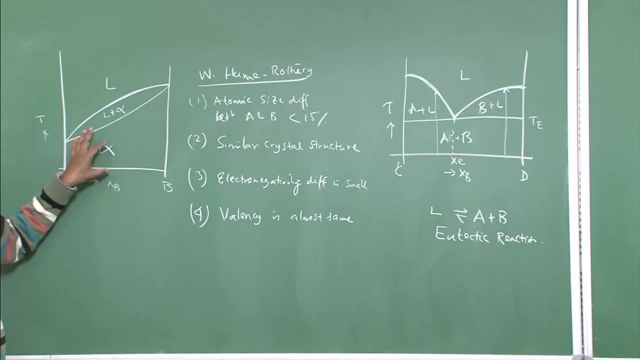 So that is why it is called easily meltable. It melts very easily at low temperature. that is why it is called eutectic. So you have understood that from this diagram, which is our isomorphous phase diagram. if these conditions are not satisfied, then we don't get these kind of phase diagrams. rather, 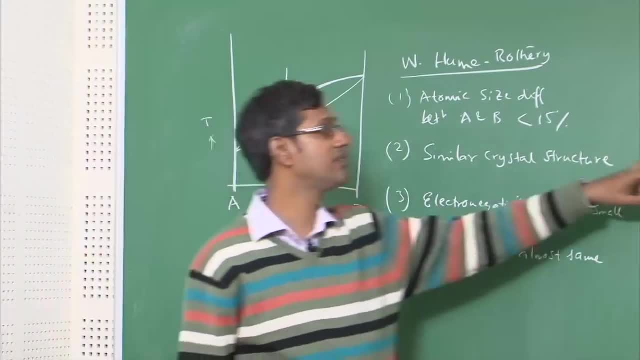 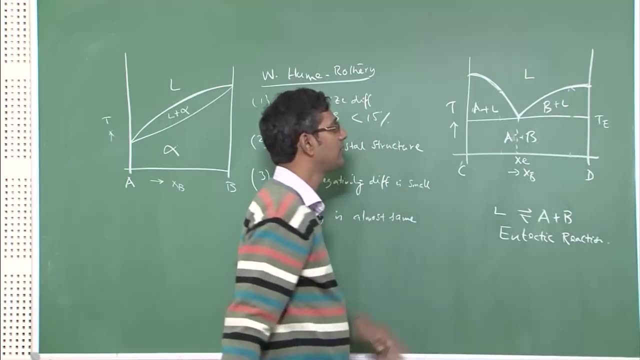 we get deviation from this phase diagrams. One such deviation is this, which is given here. This deviation is eutectic 1. In which what happens, What happens, This deviation will go and when the非常 TL adapter will. in which there is a dip in the liquidus temperature and the dip corresponds to eutectic reaction. 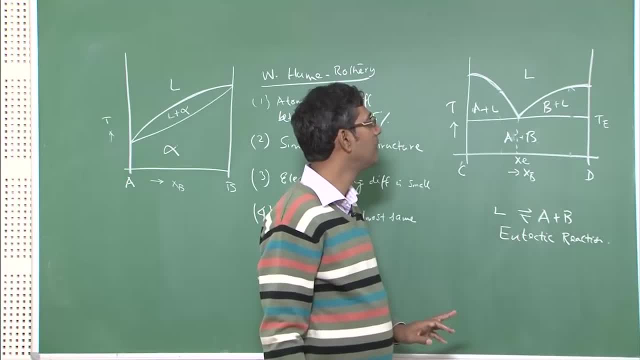 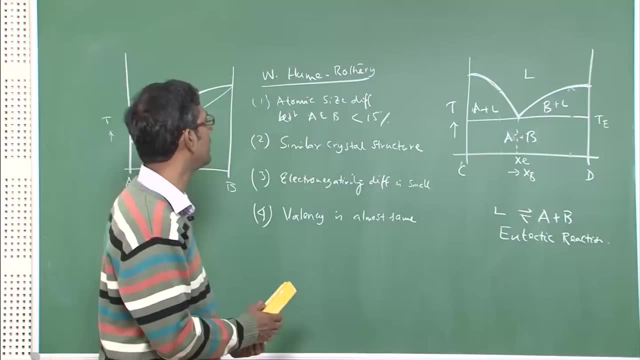 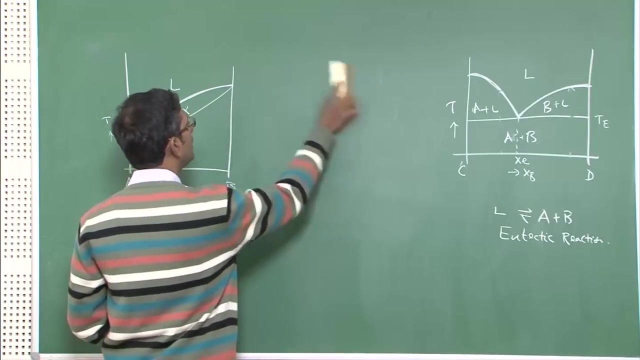 which is given by liquid, going to A plus B. So I hope this is clear. and this type of phase diagrams are known as eutectic phase diagrams in the literature because eutectic means easily meltable. that is why it is known as eutectic phase diagram. 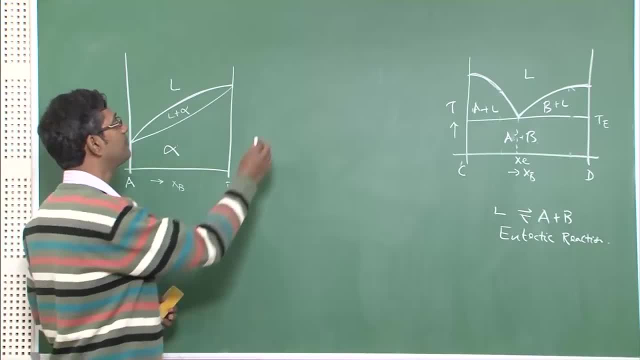 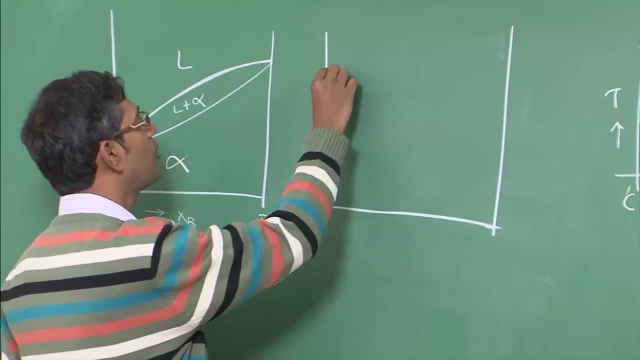 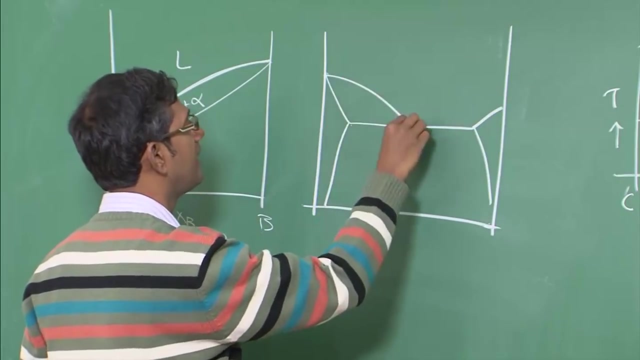 So now the most general phase, the eutectic phase diagram, will be like this. We will discuss each of these separately, you do not need to worry about it. The most general one will be like this, and it will have again a dip in the liquidus temperature. this is the liquidus. 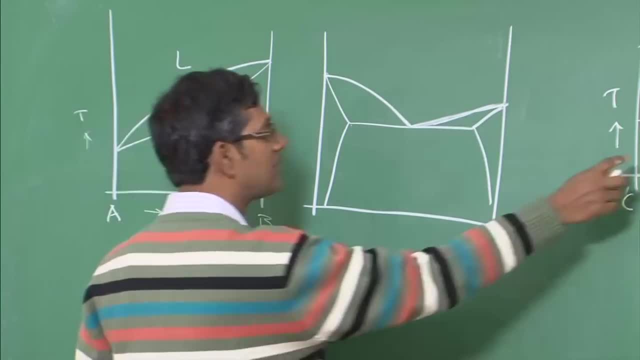 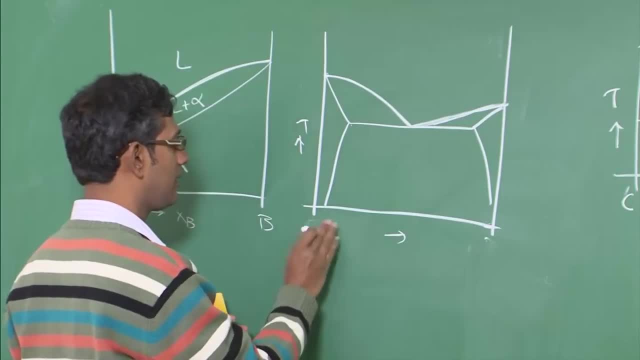 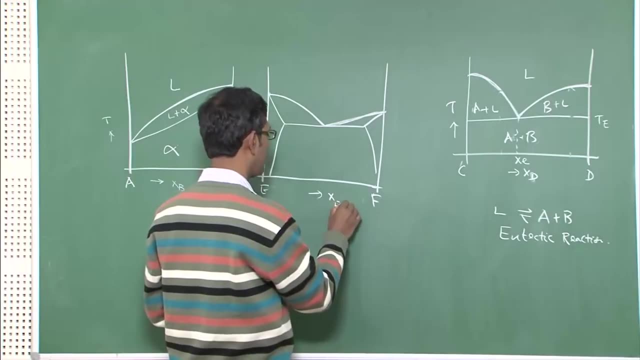 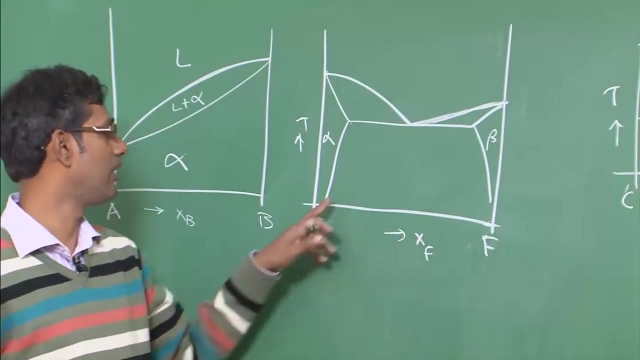 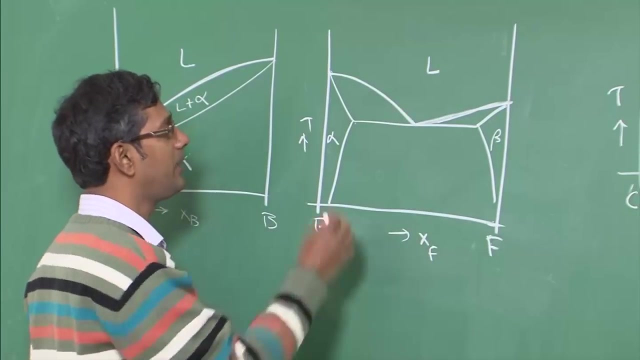 So this is not AB. these are like. these are E and F, X, F. The difference between these and these are there. There are two phase fields at the ends, end corner, at the E reach and F reach, part given by alpha and beta. This is obviously liquid, So therefore this will. 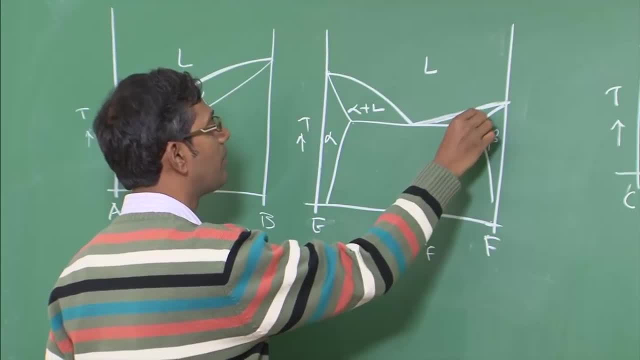 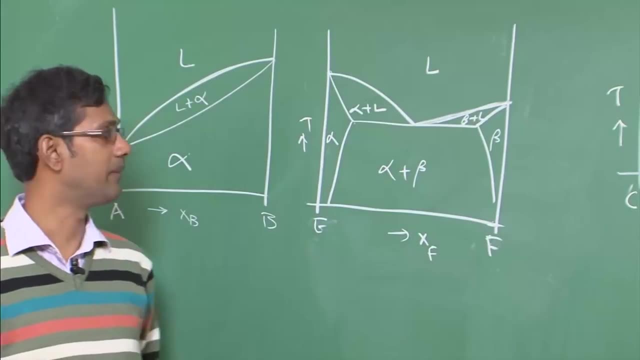 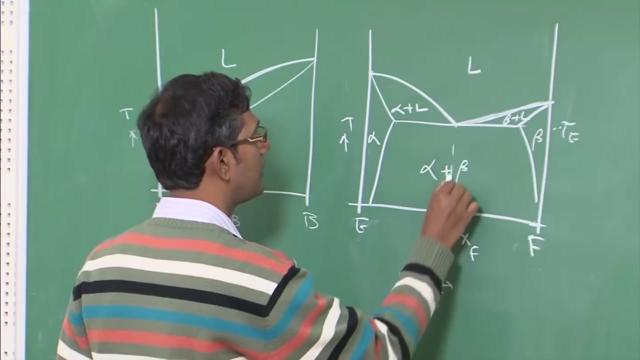 be given by liquid plus alpha, and this will be given by beta plus liquid. This is obviously. and then we have a phase field between beta and alpha, alpha plus beta. So here again, the eutectoid reaction is given by. this is Te, remember, this is Xc eutectoid reaction. 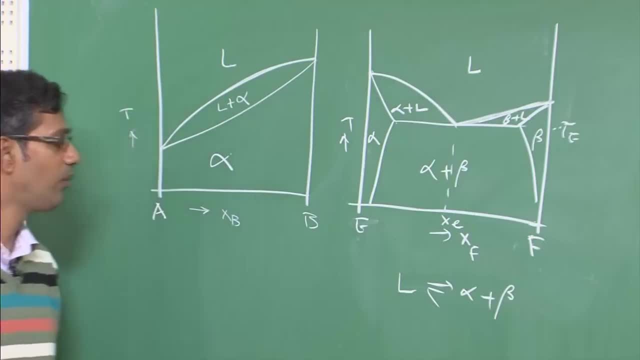 is given by liquid going to alpha plus beta While cooling. while heating this will melt like this, but we are not interested while heating, we are only interested while cooling. So this diagram will degenerate into this and from there we can get into this That 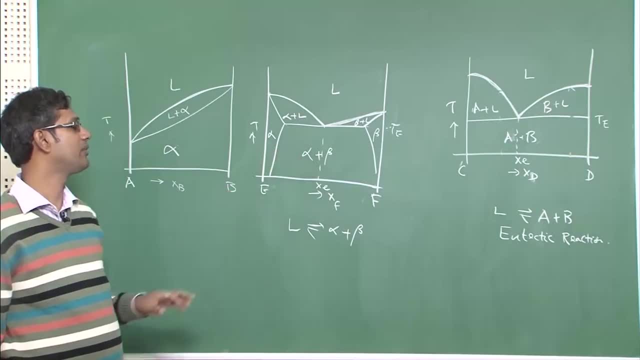 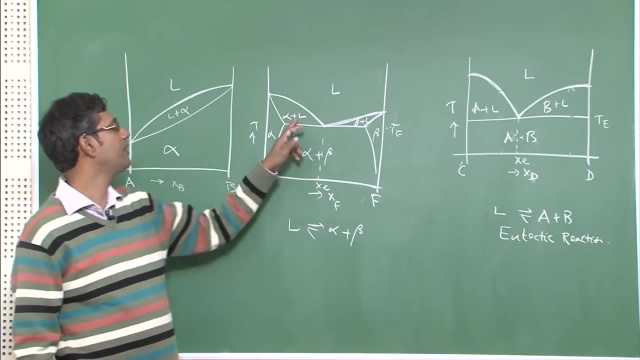 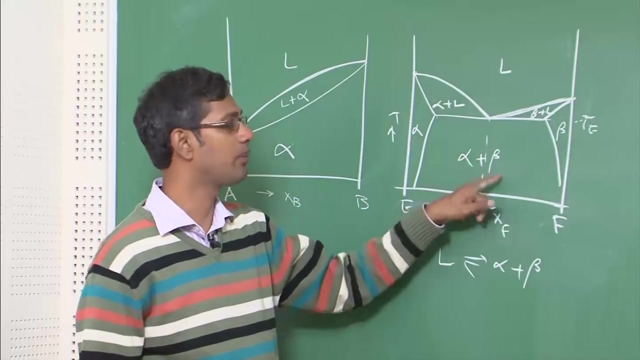 is what actually the common, most common phase diagram, a binary phase, eutectoid phase diagram in the literature will find okay. So I just explain in in details manner. here you have 1, 2,, 3, 2 phase fields: liquid plus alpha, beta plus liquid, alpha plus beta and 1, 2,. 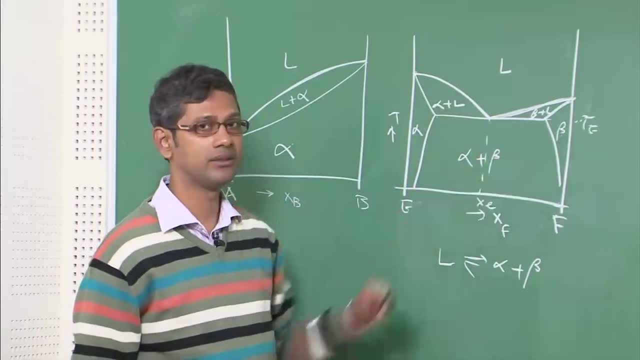 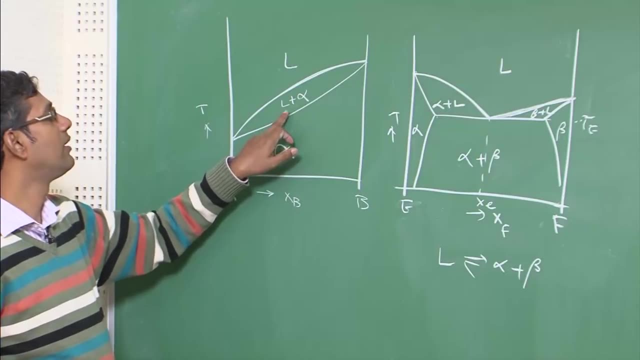 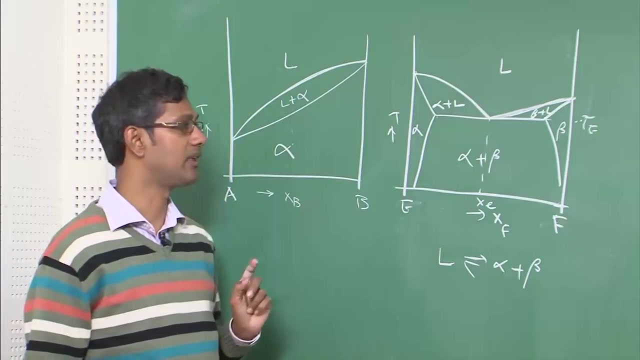 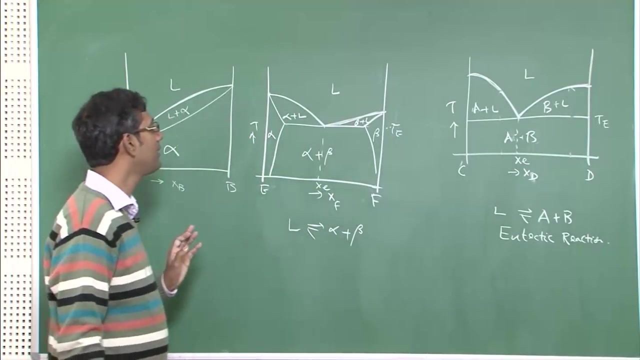 3 single phase fields- liquid alpha and beta beta. here we have one two single phase fields and two and one two phase field. so, as compared to this, we have three single phase fields here and three two phase fields here. on the other hand, here we have three two phase field and one single phase field. okay, but anyway. 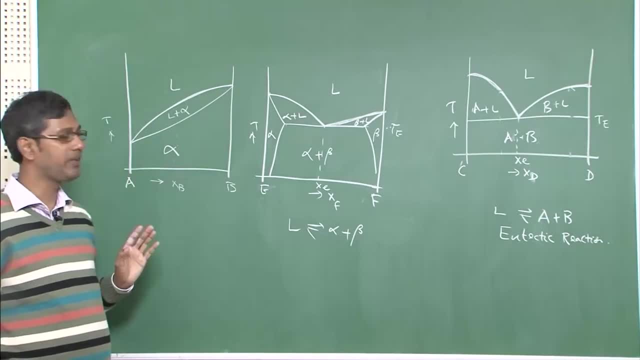 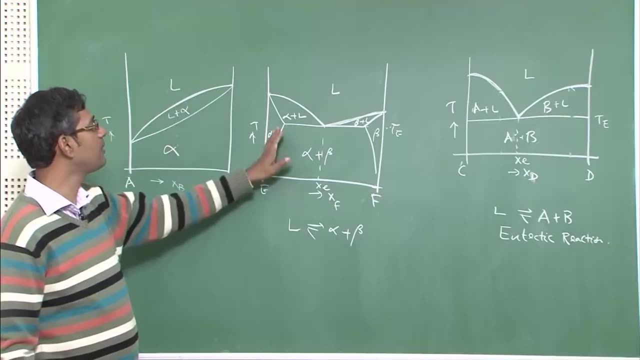 from there to here. the most important increase is the number of two phase fields: alpha plus liquid plus liquid. alpha plus beta is three. here it is only one. so that is the major difference from binary isomorphous to the binary eutectic systems. 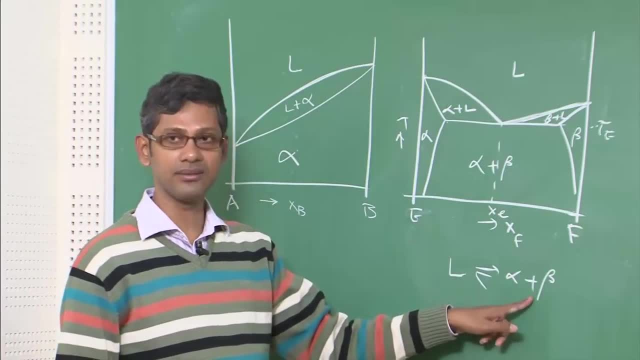 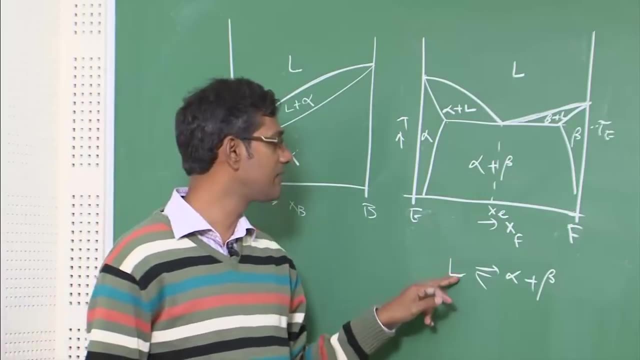 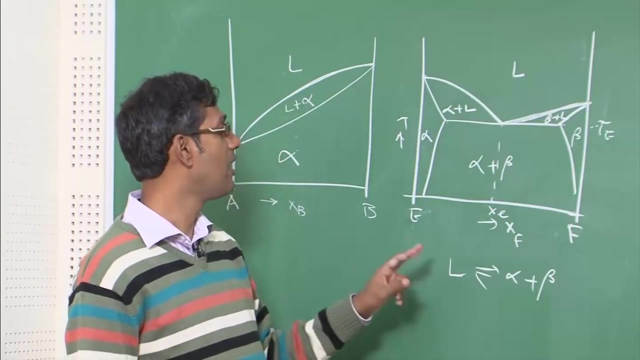 Second important difference is that in this system we have a reaction, whereas there is no such reaction happening here. here, liquid slowly becomes solid alpha, but here, in this case, liquid undergoes a reaction and produces two alpha simultaneously. please remember this word: simultaneously, Liquid transforms into liquid. 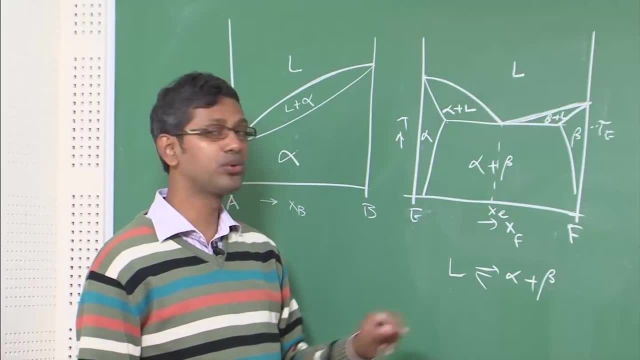 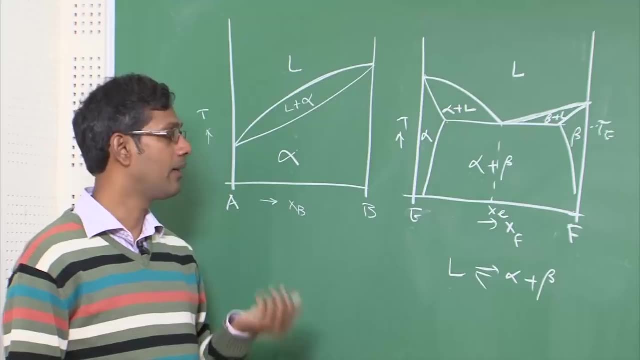 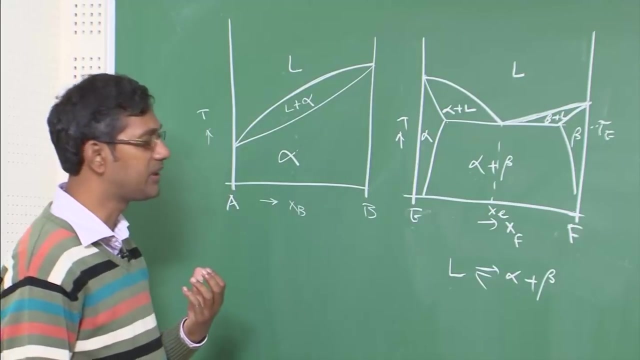 Liquid transforms into two solids simultaneously and these two solids coming together leads to different kind of microstructures or different kind of microstructure features that we are going to see today itself. So my basic point I want to trace upon is that, because of this reaction, we have a large 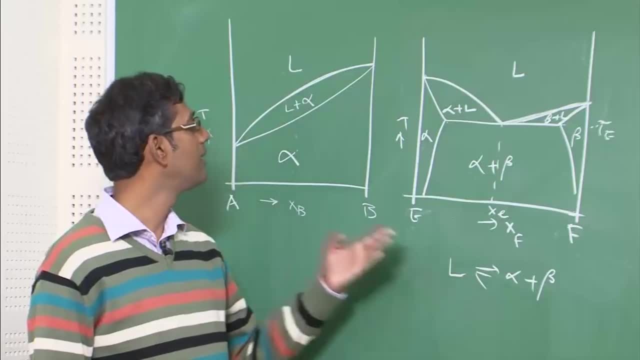 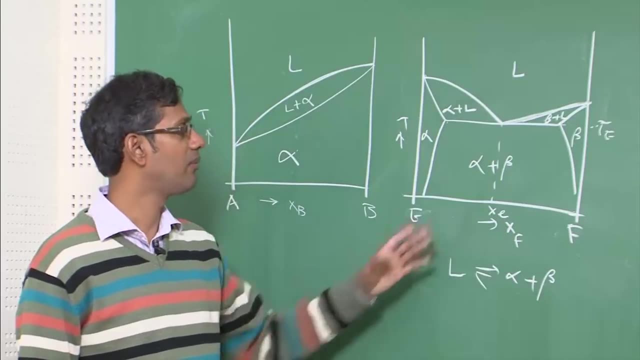 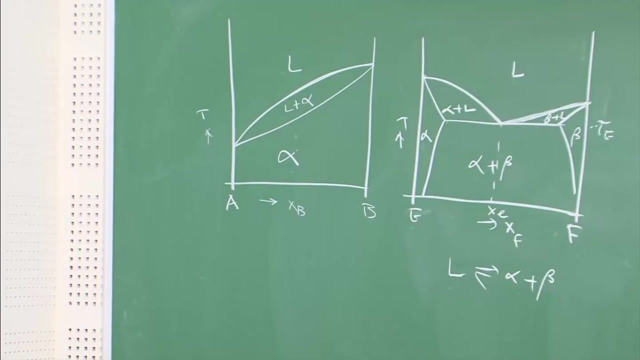 number of different kinds of microstructure development, whereas here we do not have that many. So that means it gives you It gives you many opportunities to control the microstructure by this reaction, which we do not get in isomorphous system. So let me just get into the different kinds of phase diagrams and tell you how it is possible. 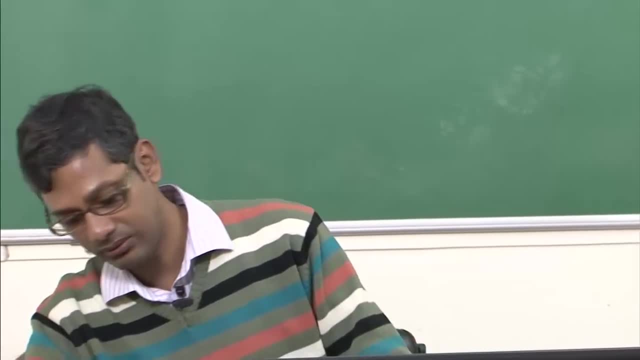 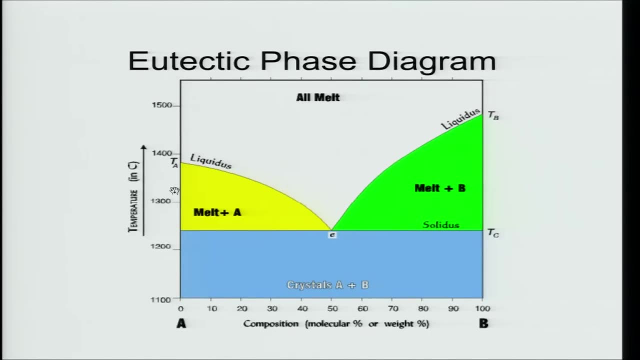 Okay, so this is the diagram I just discussed right now. okay, this is the diagram I just discussed right now. you can see here, this is the simplest possible diagram, in which A and B are the two components. it can be anything. Okay, So this is probably in the A2, which is the first phase. 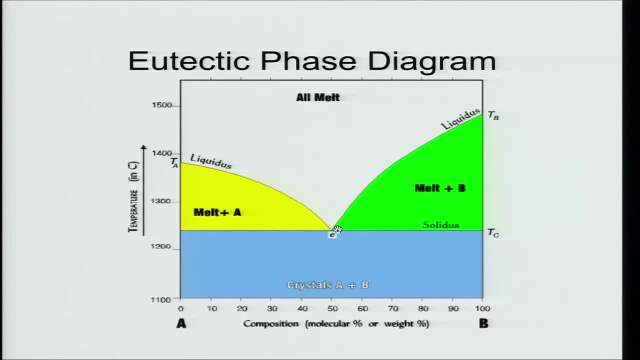 This is the second phase in the B1, and the third phase is the third phase, where we have two impurities and one impurity here, and this Y decision is the fully liquid decision and then you have a liquidous. these two are the liquidus one coming down for military temperature. 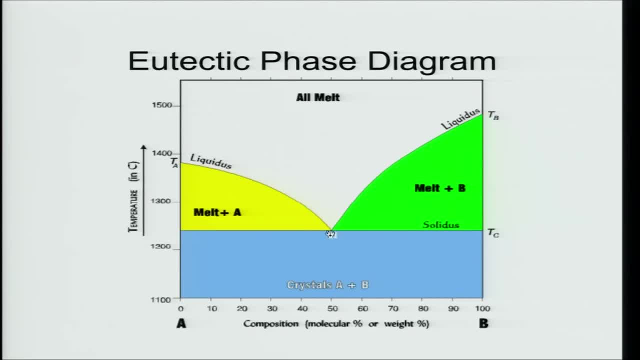 pure A, other one coming down for military temperature, pure B. and they meet at a temperature, at a concentration E. they meet at a concentration E and temperature Te. that is why the utility temperature and utility composition, and therefore this yellow color phase field, is liquid plus a or melt plus a. 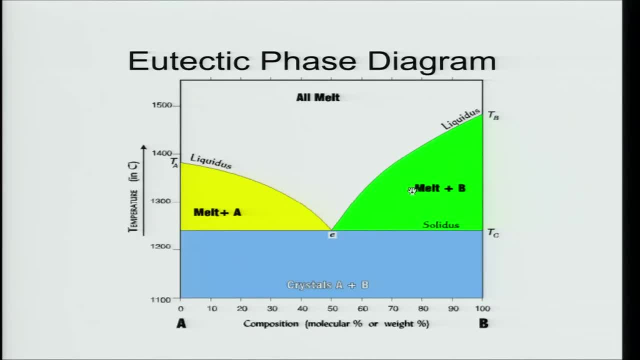 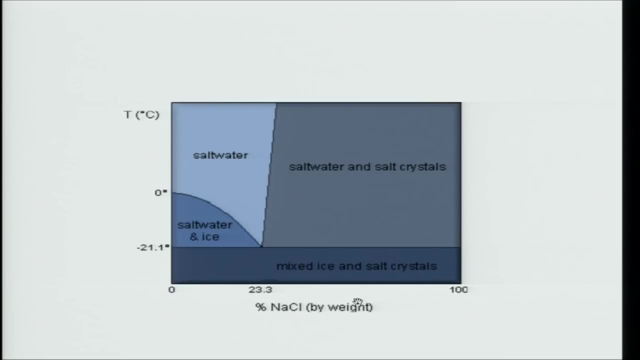 Yes, On the right side, green color phase build is liquid plus B and you have at the bottom above, below the eutectic temperature, you have crystals of A and B, rather A plus B. This is the common phase diagram between sodium chloride and water and it has very interesting. 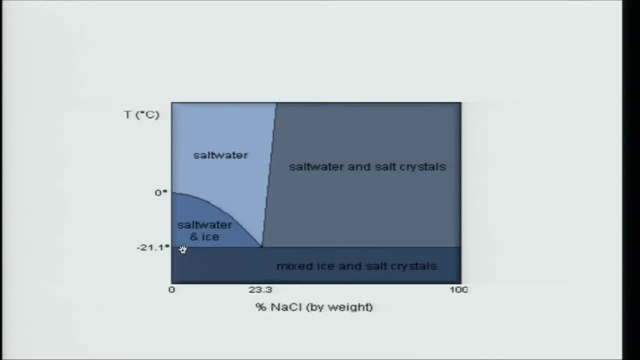 implication. If you look at this diagram, eutectic temperature for sodium chloride and water, this is pure water. this is pure sodium chloride. right side is pure sodium chloride and you can see as you keep on adding sodium chloride, at about 23.3% of sodium chloride concentration. 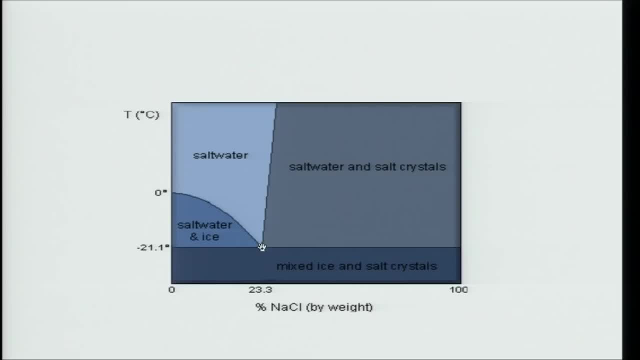 you have a dip in the liquidus, and this dip corresponds to eutectic temperature, which is given by minus 21.1 D Celsius. This is the reason. in the northern hemisphere, when there is a snowfall, in order to melt the snow, people add sodium chloride. 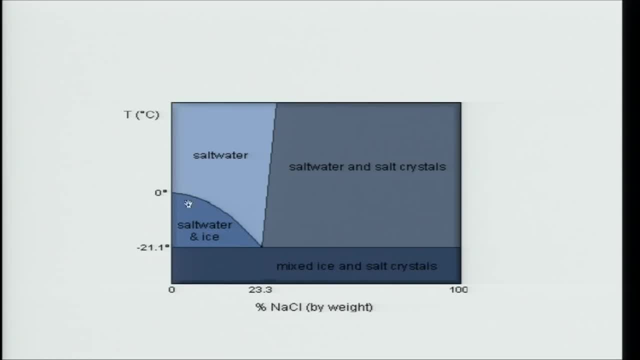 Why? Because snow normally melts or ice normally melts at 0 D Celsius or above, but if you add sodium chloride into it, the melting temperature goes down to minus 21 D Celsius temperature. So that means you can easily melt down the ice or snow by adding sodium chloride and 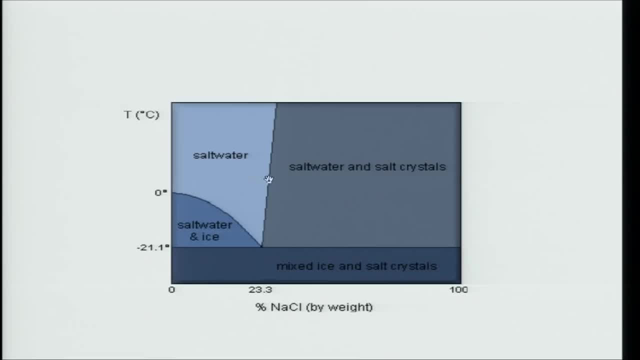 you can understand these things by using eutectic phase diagram. This is the beauty of eutectic phase diagram. At a concentration of sodium chloride of 23.3 weight percentage at about minus 21 D Celsius temperature, This is the eutectic reaction in which salt water, while cooling, transform into mix of 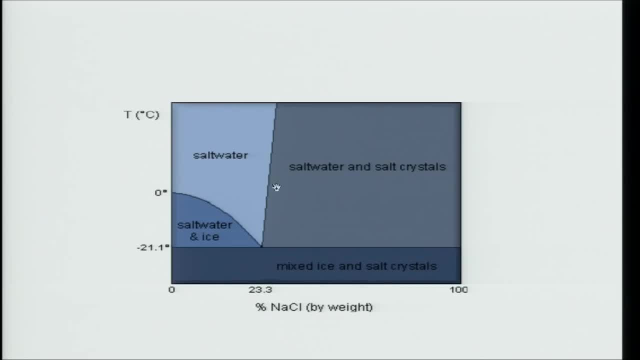 ice and salt crystals. So that means, if I heat it up beyond 21 D Celsius temperature- a mixed ice and sodium salt crystals- they will become water. So that is what you want. We normally want to melt the ice in the northern hemisphere when there is a huge snowfall. 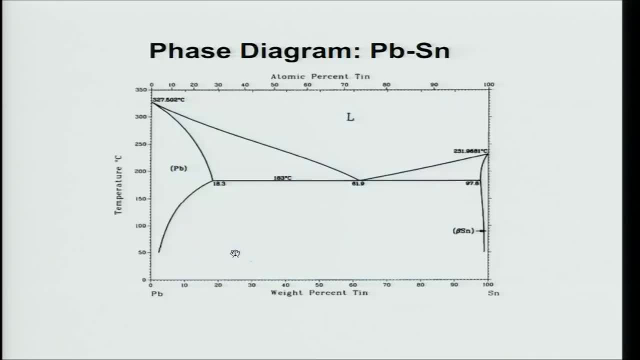 So we sprinkle- that is why sodium chloride or common salt, into the water. Now, the most common reaction, Now the most common reaction, The most common phase diagrams of the second one, which I discussed in the blog, in which there are two end phase fields, one is alpha and one is beta- is the lead tin solder. 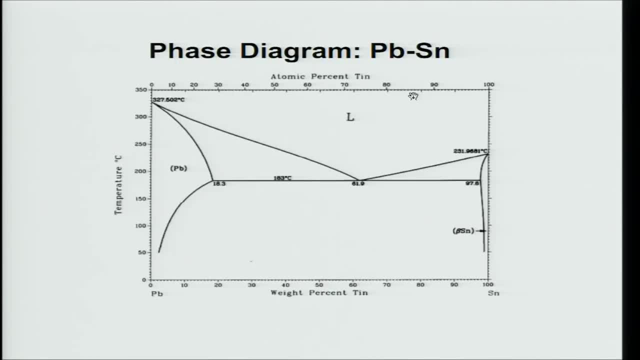 Lead tin is a very classic example of eutectic system. Why? Because lead tin alloys are used to make solders in the any kinds of device you want to make, whether it is a computer, it is a mobile phone or it is anything. the soldering element is 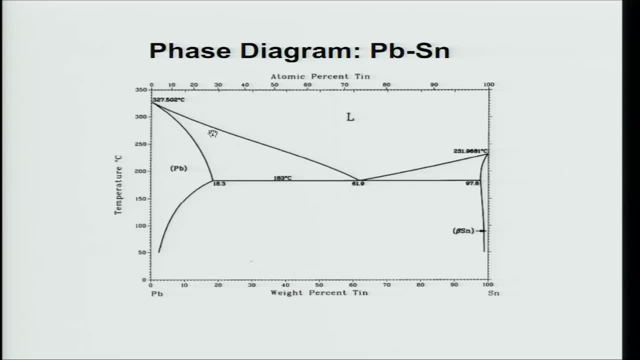 lead tin alloy- Lead tin alloy- Okay, And if you look at this phase diagram, lead tin alloy at about containing 61.9 weight percent of tin. it melts at 183 D Celsius temperature. this is the melt temperature, Okay. 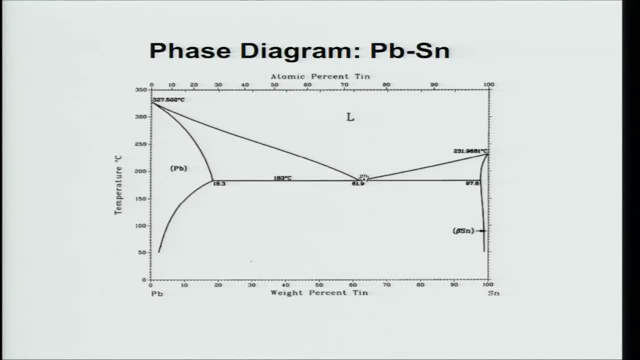 So that means it melts at a much lower temperature. We can easily join or solder two pieces of coil or cable in the electronic device. That is why this is widely used as a solder material in the electronic device And it is very important. So now this is a classic eutectic phase diagram, the second type I showed you where we have 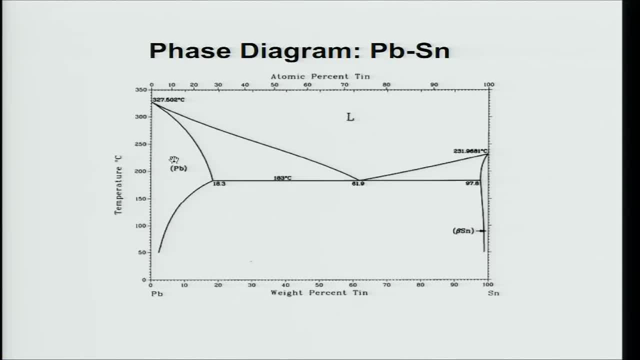 two ends. one is lead tree chain, other one is tin tree chain. you have a lead solid solution, known as alpha or PV, within first bracket, and on the right side you have beta, tin solid solution within first bracket: beta, tin or beta, whatever you define. 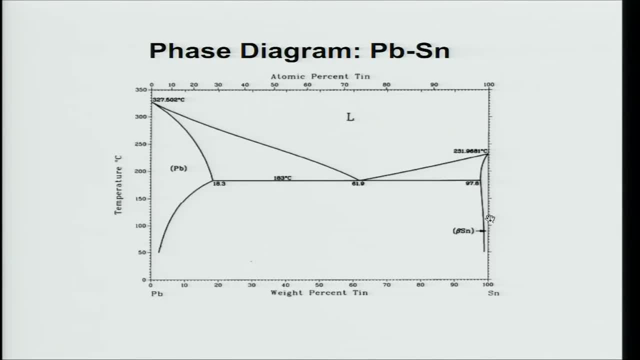 By the way, tin exists in two forms: alpha and beta. Okay, So this transformation happened at 281 Kelvin and this is a very important phase transformation for many of these historical perspective which I will discuss maybe later. But so these are the two ends, which are solid solutions, just like binary isomorphous systems. 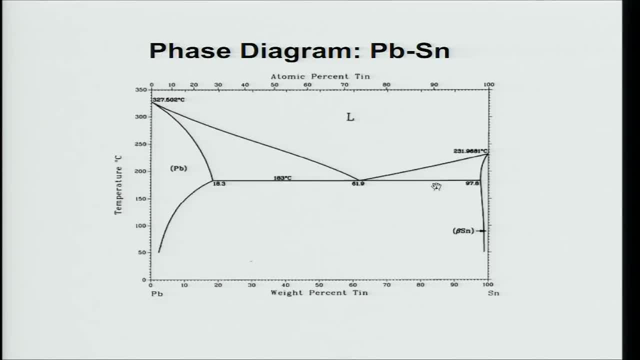 and between that we have a binary, we have a binary eutectic phase diagram existing. So therefore this phase field which I am showing here is basically liquid. Okay, This one is liquid plus alpha, this one is liquid plus beta and this one is alpha plus. 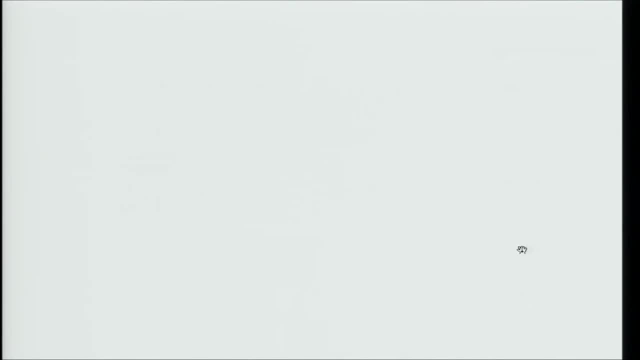 beta. Alpha is lead solid solution, beta is tin solid solution. Okay, So now, upon knowing this, let us now discuss little bit more, and because this is very important, and I just go back to board and explain you this stuff, Okay, So, as you see here, I have kept the phase diagrams nicely. 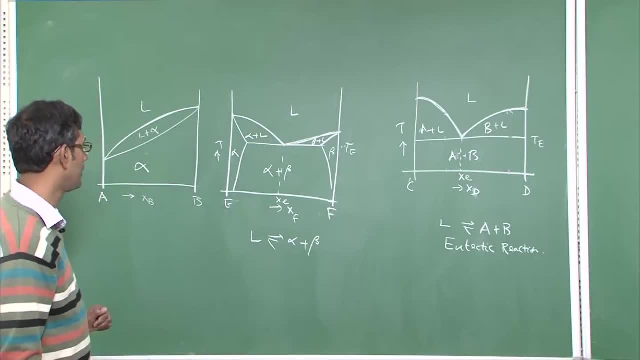 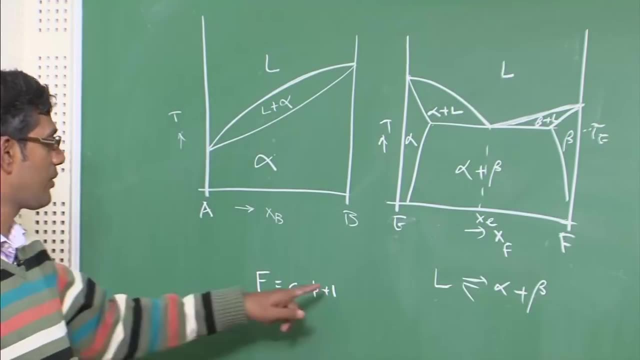 So now let us consider and apply: phase rule gives phase rule here. Okay, So the Gibbs phase rule is given by. F is equal to C minus P plus 1 when pressure is kept constant. That is why 1 comes. Remember when pressure and temperature both are varying, then it will be 2.. 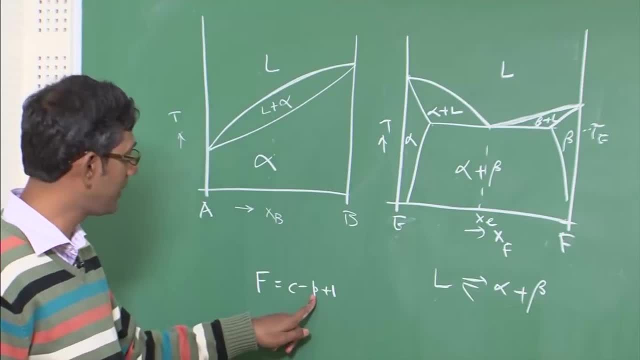 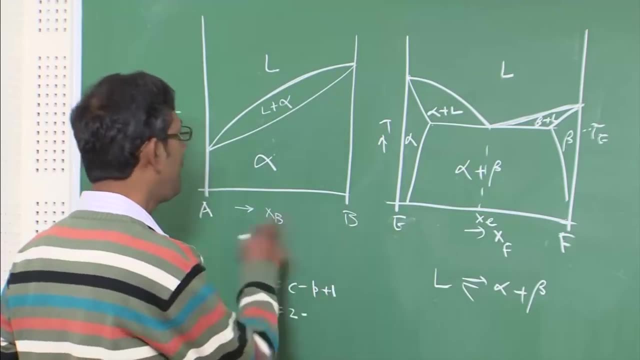 So C is small, c is the number of components, P is the number of phases and F is the degree subsystem. So here C is equal to 2, because it is a binary system: A, B or E, F or C, D. there are two components. 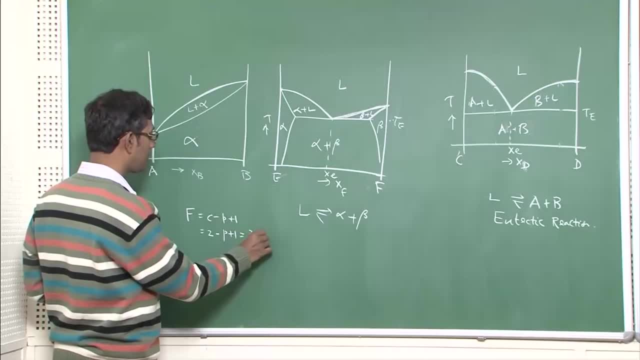 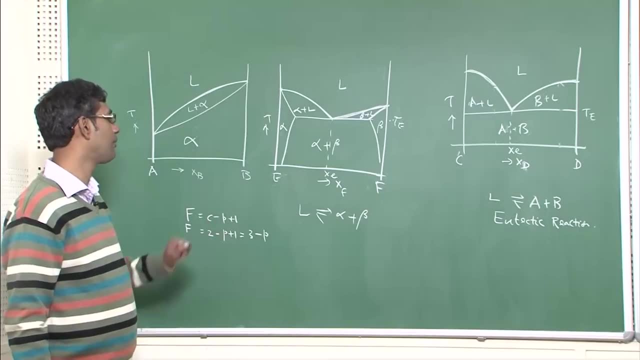 So there are two components: 2 plus minus P plus 1 is basically 3 minus P. That is the value of F. Okay, I hope it is clear. C is number of component 2, P is the number of phases. 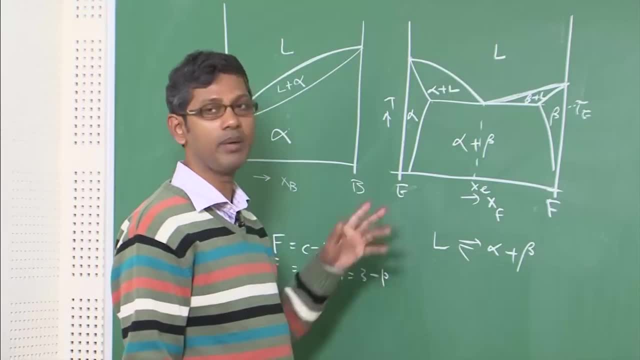 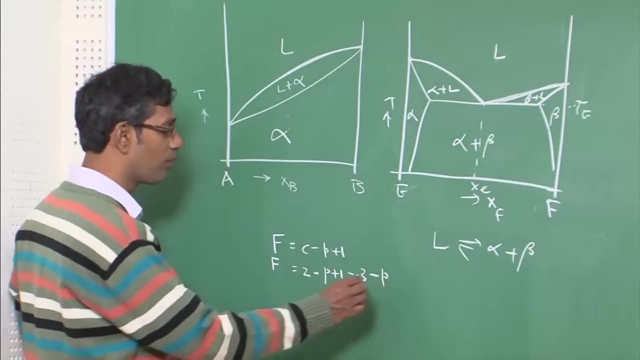 Now let us apply this in single phase fields of these binary utility systems. There are 3, alpha, beta and liquid. So you have a single phase field, that is when P is equal to 1,. if P is equal to 1, then F. 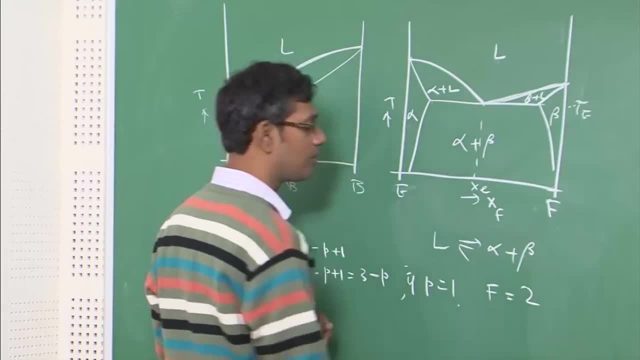 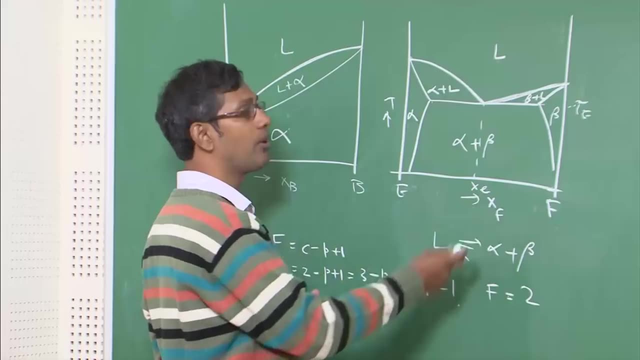 becomes 3 minus 1, 2.. So what does it mean? I explain you. in this case, That means I have 2 degrees of phase. That means I have 2 degrees of freedom. That means I can vary both temperature and compositions, but I will be in the same phase. 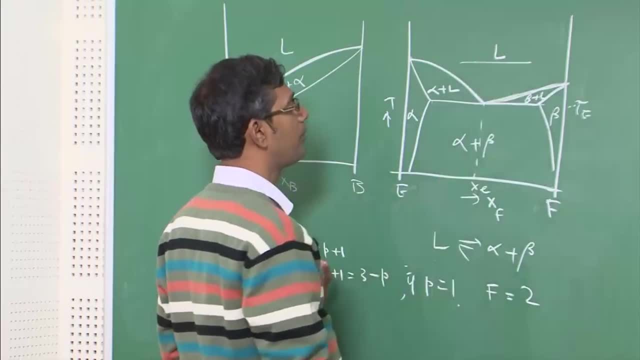 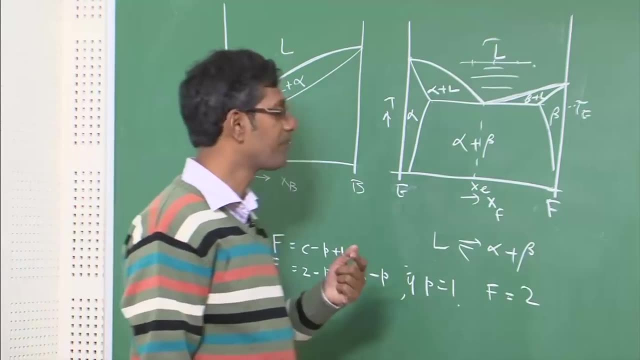 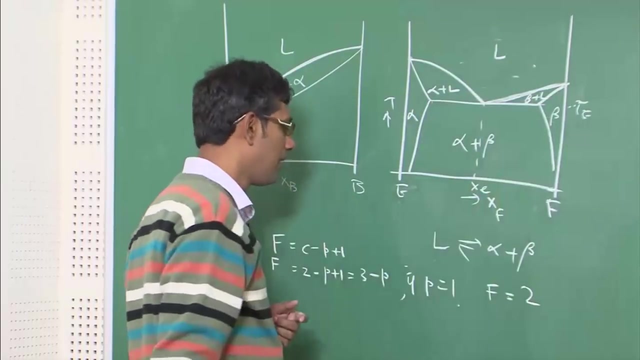 field. You can take any point here. you can buy the compositions or you can buy the temperatures, like this, but still you are in the same phase field. So that is what is the case for again, alpha and beta. Same thing will happen between alpha and beta phase field. 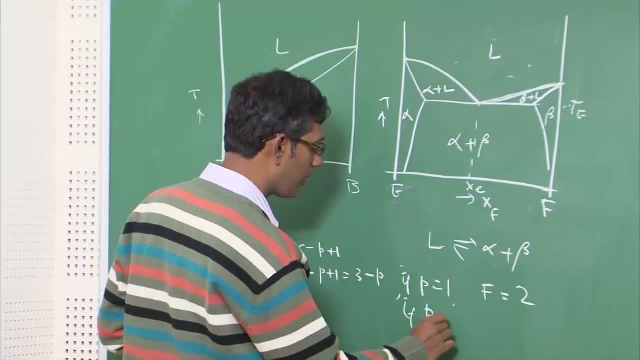 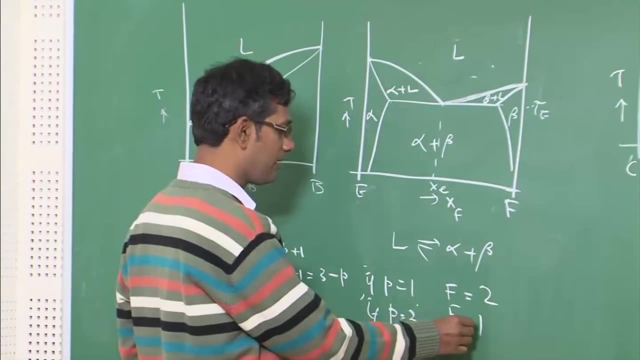 Now, if P is equal to 2, what will happen? F is equal to 1.. 3 minus P, 3 minus 2 is equal to 1.. If F is equal to 1, what does it mean? That means the degrees of freedom is equal to 1.. 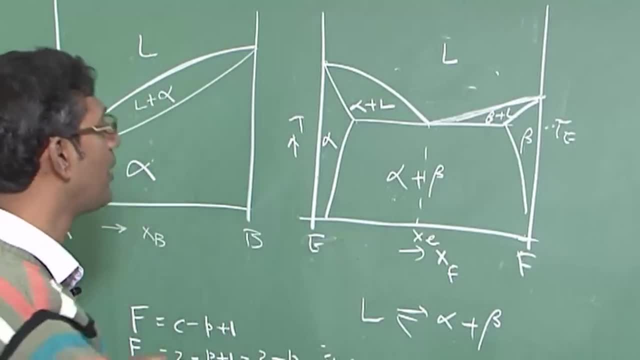 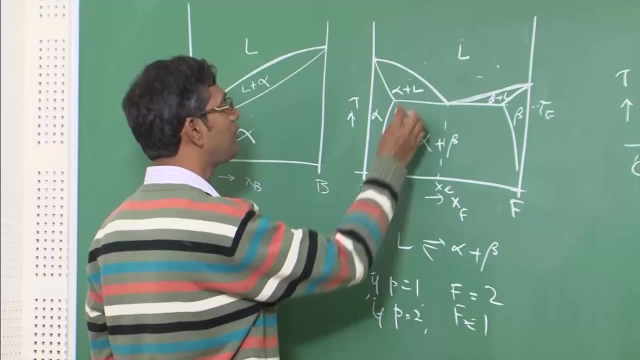 So if I go to the 2 phase field, suppose alpha plus beta, and let us do it for alpha plus liquid, Suppose if I go here Now, if you can see that if I choose a composition, suppose I choose a composition X1.. 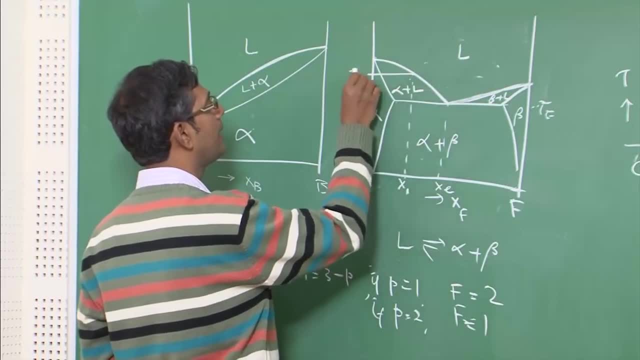 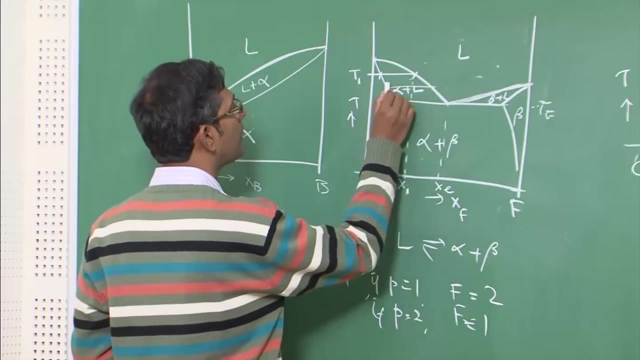 So now I can clearly see that at X1,, at any temperature T1, my composition of 3 is equal to 1.. The composition of solid and liquid are fixed. Similarly, at any temperature T2,, my composition of solid and liquid are fixed. 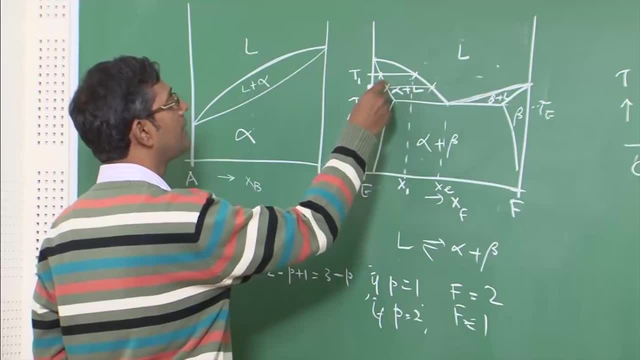 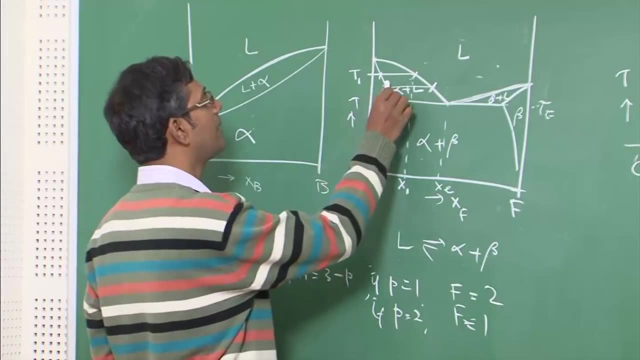 These two are the. this is a tie line connecting soliders and liquiders for the solid composition given by this Liquid composition given by this- I have explained you already- I draw a tie line in temperature which connects the two soliders and liquiders. 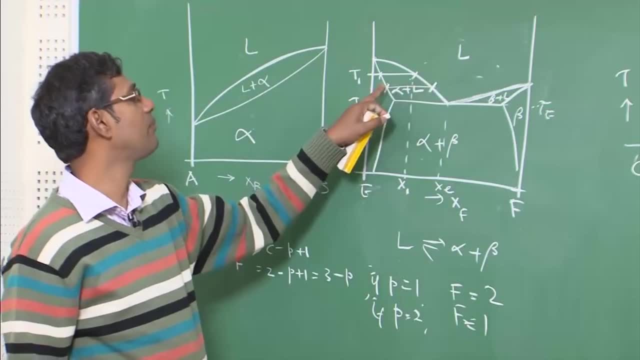 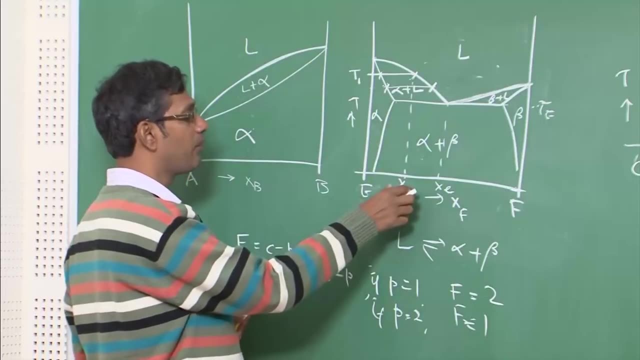 The cross section points will be the composition of solid for the soliders, liquid for liquiders. So what I mean to say is that if I choose a composition, I have composition I choose. I do not have any freedom of choosing the temperature, because 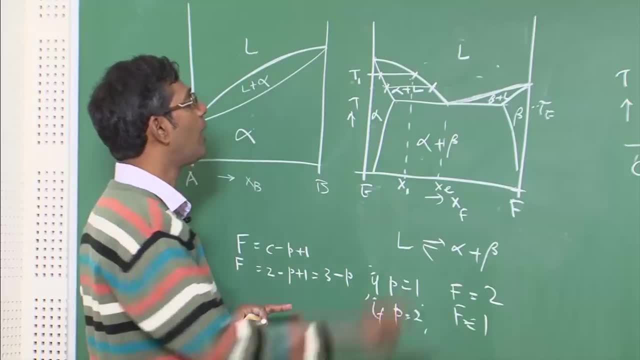 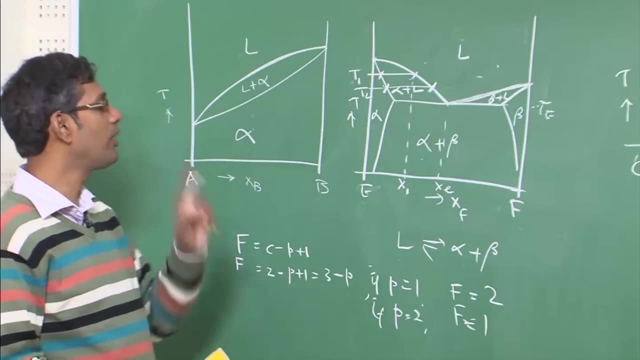 composition of the solid and liquid are given or if I choose a temperature- suppose this one- T2,- composition of solid and liquid are fixed. So either way, I have only one freedom: I can either choose a composition or choose a temperature. I cannot choose both of them together. 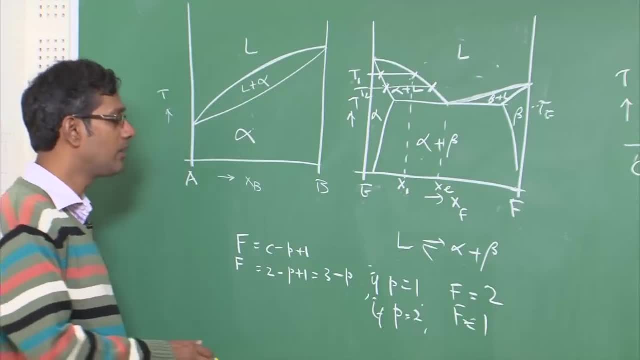 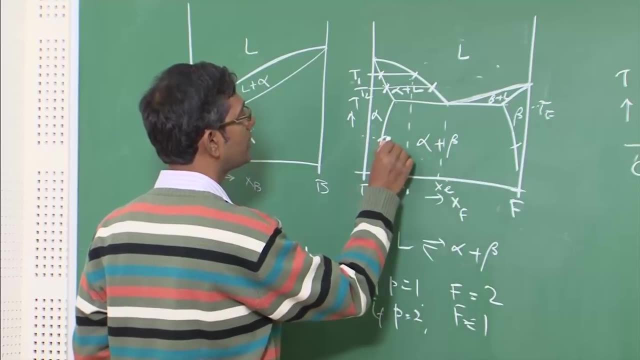 If I choose, then I will be getting out of the 2 phase field. Now the classic thing will come, and this is same thing for alpha plus beta. I choose the compositions. this or I choose a temperature. You can see here: the compositions are given by these two lines. 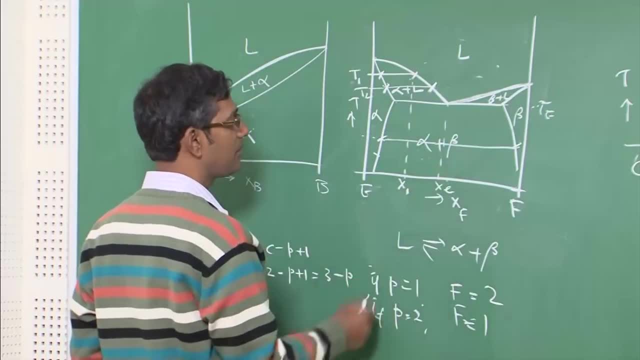 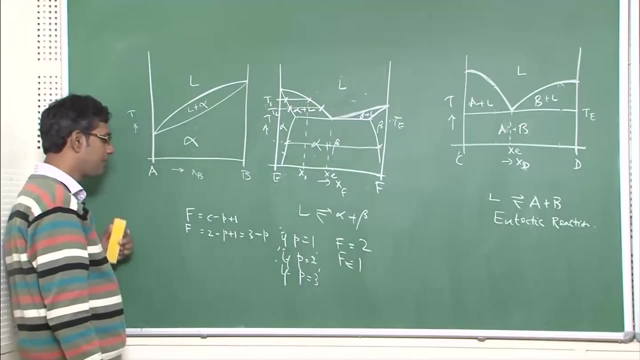 And if I choose a composition also, the temperatures are given. temperature will be fixed. But classic thing will come if I consider pressure to be P to be 3. If P to be 3 means F is equal to 0.. P means number of phases. 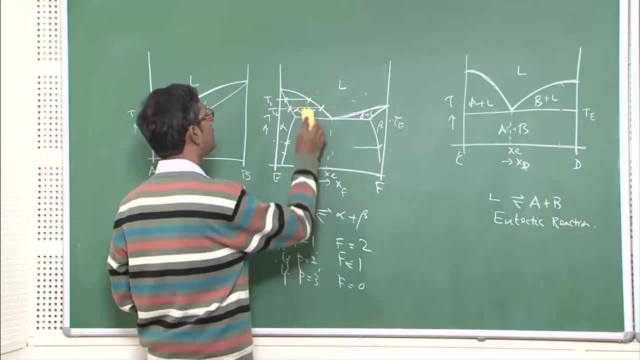 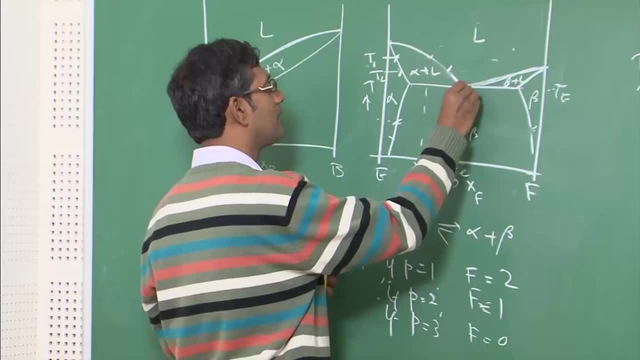 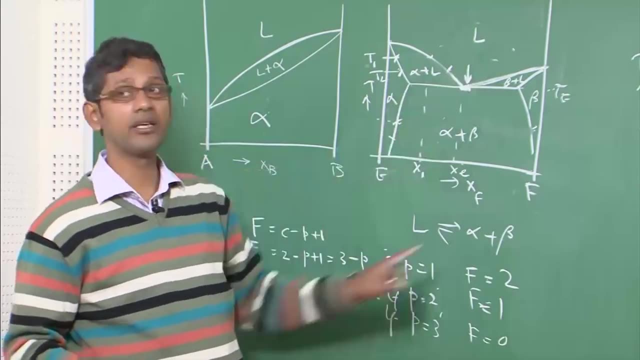 What is that correspond to? That correspond to this point. At this point I am marking by arrow. At this point, all the 3 phases- alpha, beta and liquid- are coexisting, and that is why P will be 3.. So that means at this point I have no degrees of freedom. 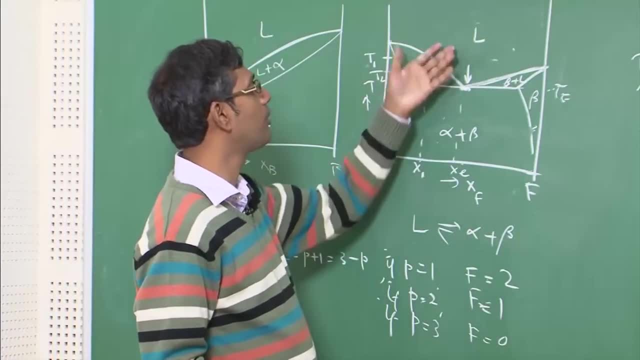 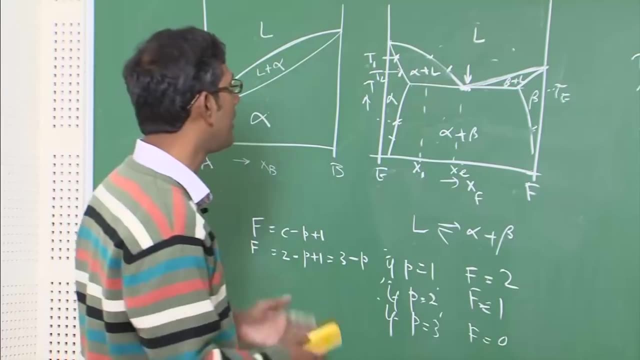 If I simply change my temperature a little above and below, I will be out of this point. Or if I change the composition a little bit this way, that way I will be out of this point. So question is this: that this point is having degrees of freedom equal to 0 and known as 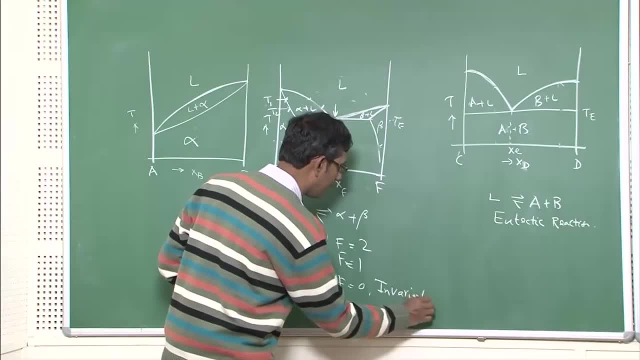 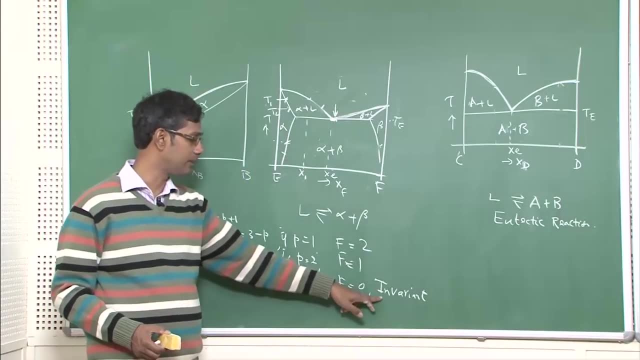 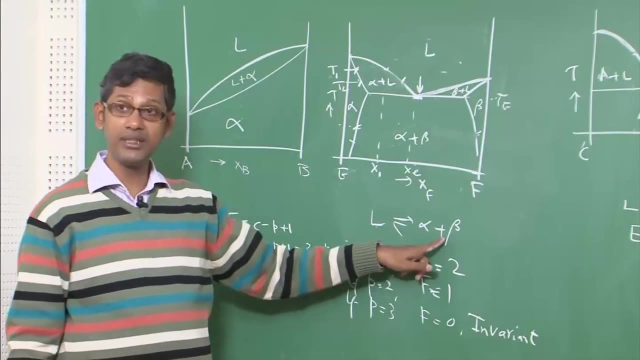 invariant point. I cannot vary anything here. invariant point. So that is the definition of an invariant point. At the invariant point you have no degrees of freedom, You have only 0 degrees of freedom. Remember any reactions which involve 3 phases, whether it is a liquid going to alpha beta. 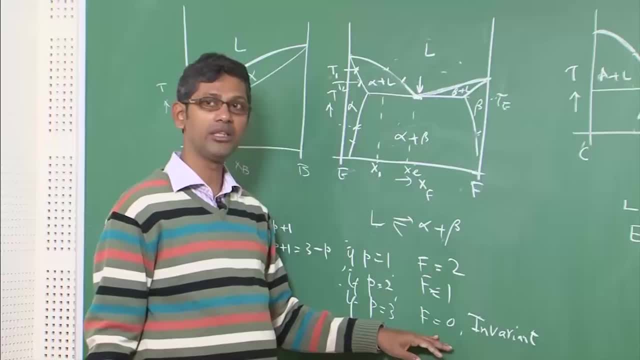 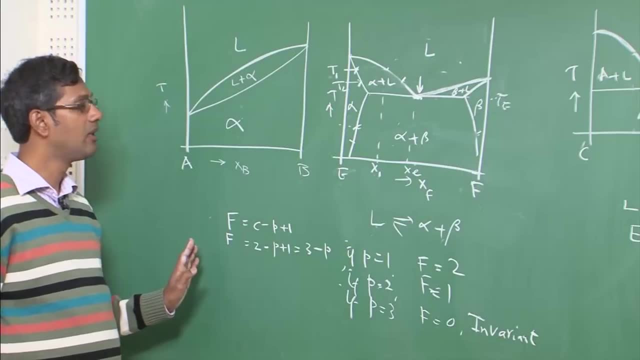 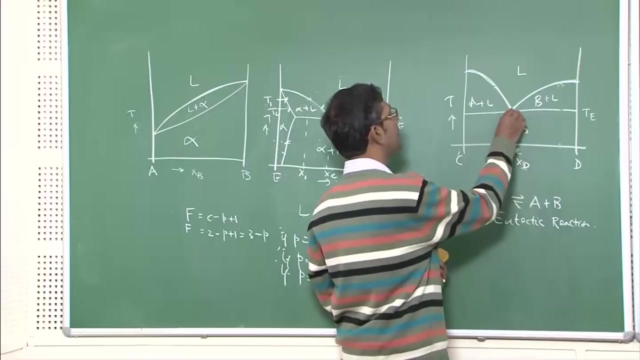 beta or any other phases. you have no degrees of freedom present. You have only 0 degrees of freedom present. This is a very important concept as far as the phase rule application is concerned. So you can actually apply phase rule here itself, here also on this point, your degrees. 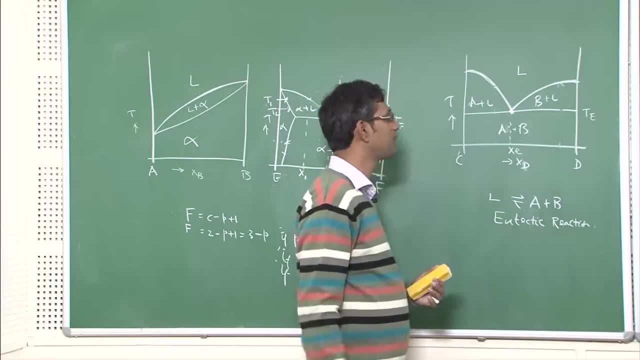 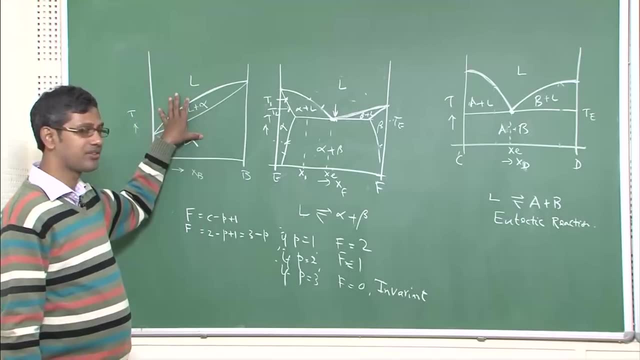 of freedom is equal to 0, and in these 2 phase fields, your degrees of freedom is equal to 1, and in the single phase field, your degrees of freedom is equal to 2.. So therefore, as compared to this, you have a 1 extension. 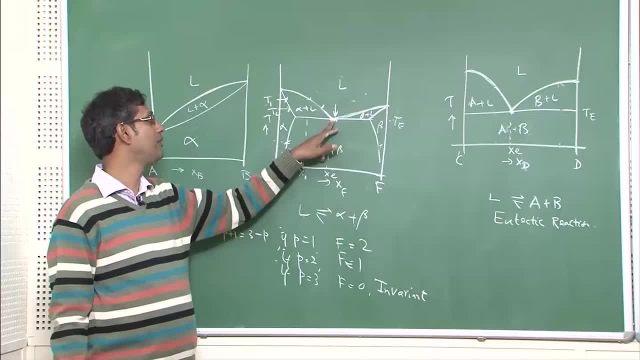 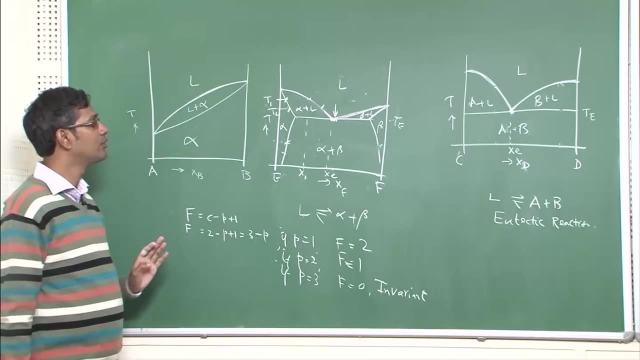 You have a 1 extra point, That is the eutectic point. At the eutectic point, you have a degrees of freedom equal to 0.. In this binary isomer phase diagram, nowhere your degrees of freedom can be 0. 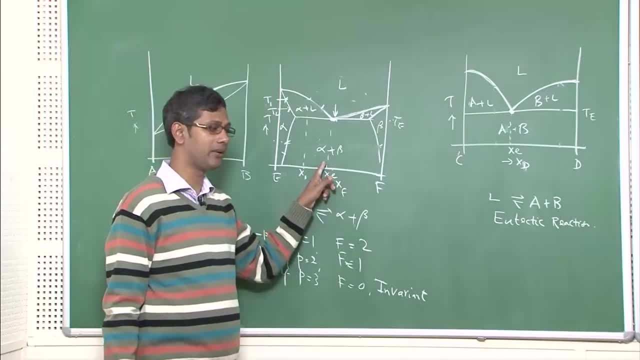 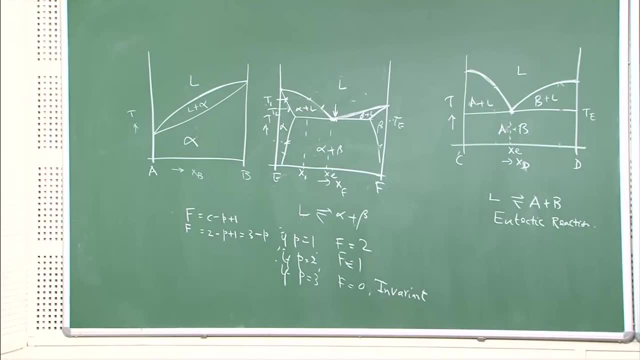 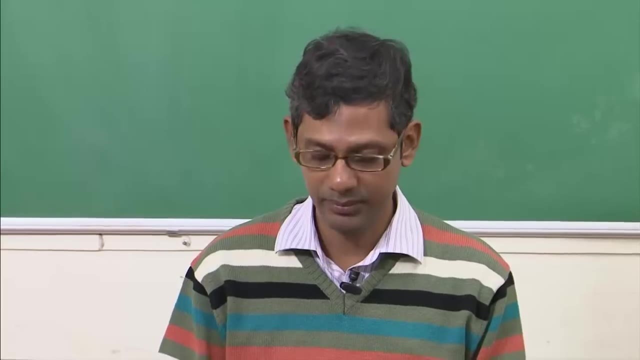 So we start seeing degrees of freedom to be equal to 0 only from a eutectic phase diagram. This is what you should remember in all your lectures. So now I think I will just discuss about the phase formations, and before I do that, because 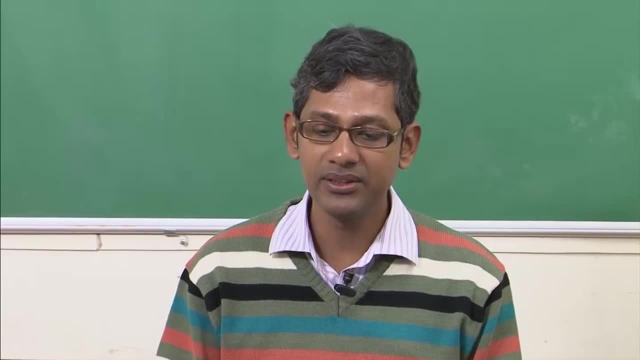 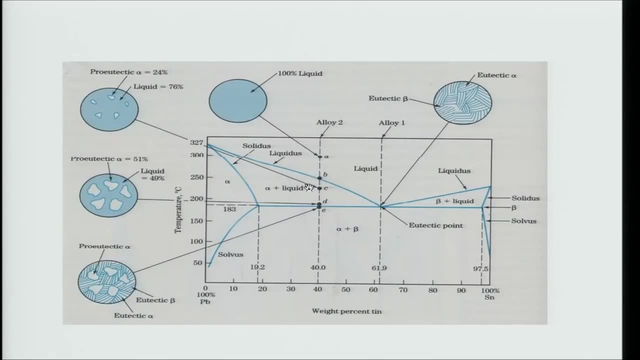 we will discuss in detail In the next class. before I do that, let me just tell you that this particular phase diagram, which I discussed late in, has there are 3 types of alloys to be present or discussed. The one which is made 1, alloy 1 is the eutectic alloy. 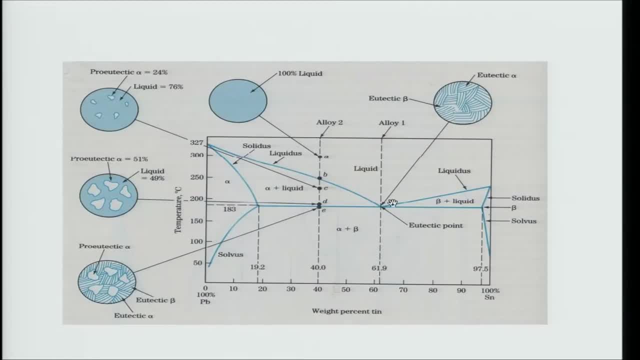 So we will discuss the eutectic alloy first. and there are alloys whose composition is less than the eutectic compositions. that means between this point- this is one point of this horizontal alloy, This horizontal line- and the eutectic point. these are called hypo-eutectic alloys.